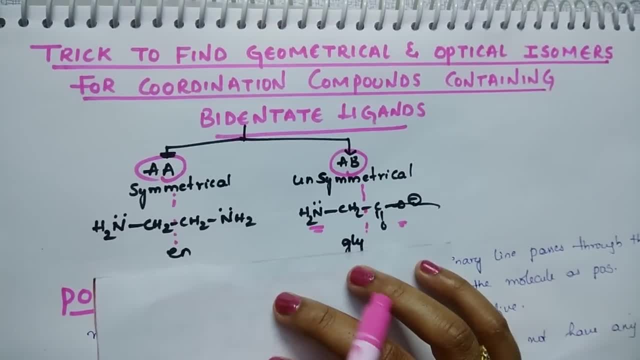 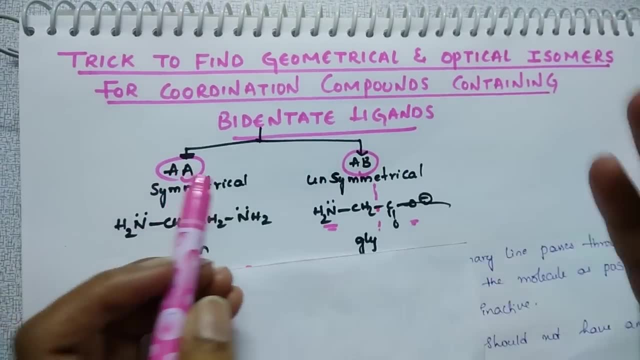 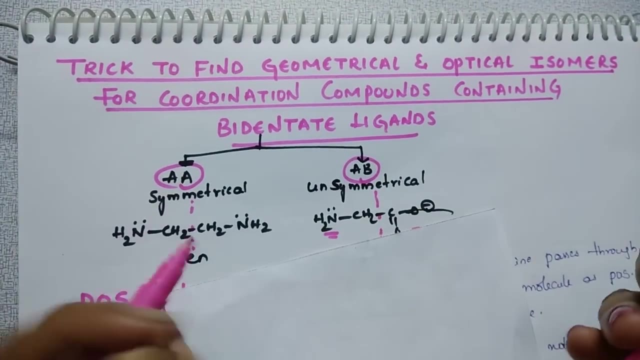 two different donor atoms like nitrogen and oxygen in glycinate molecule, then we call it as unsymmetrical ligand Means two types. what are those? AA type and AB type. See here to understand this. if in line, imaginary line passes through this molecule, if you get two equal halves. 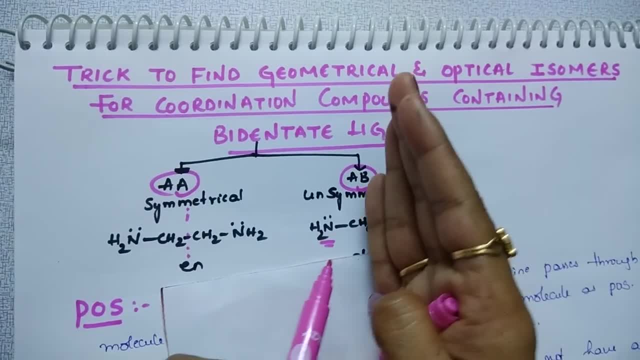 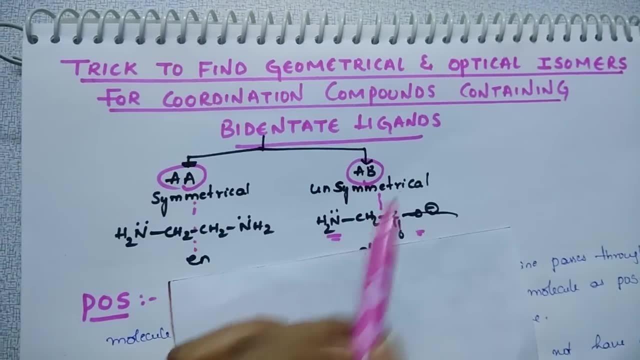 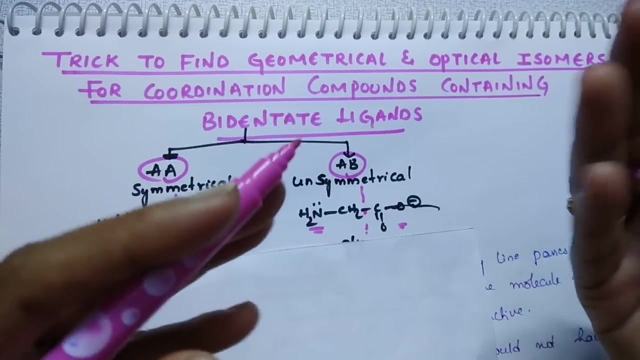 then we call it as symmetrical. If imaginary line passes through the molecule, then we get two different here, different here also here also different. then we call it as unsymmetrical ligand. To find the geometrical isomers: what you should do is you have to find the number of. 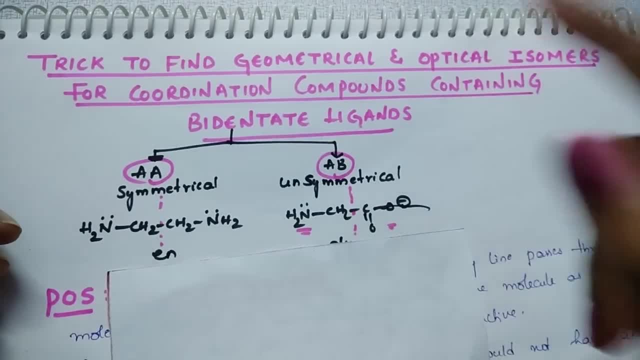 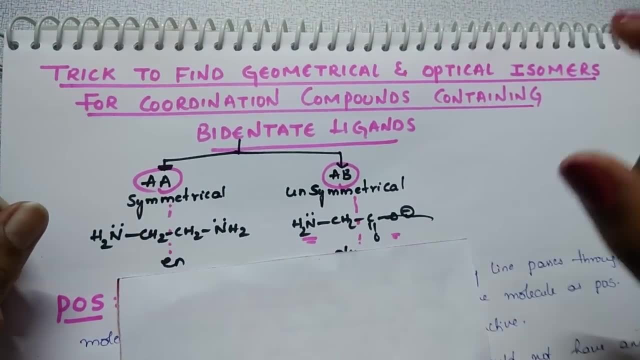 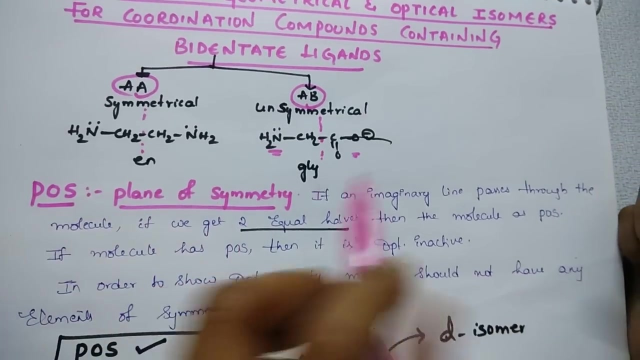 combinations possible. Is it clear What you should do? You should find the number of combinations, Combinations possible and to find the optical isomers, You should see whether the particular coordination compound is having plane of symmetry or not. What is this plane of symmetry if an imaginary line? 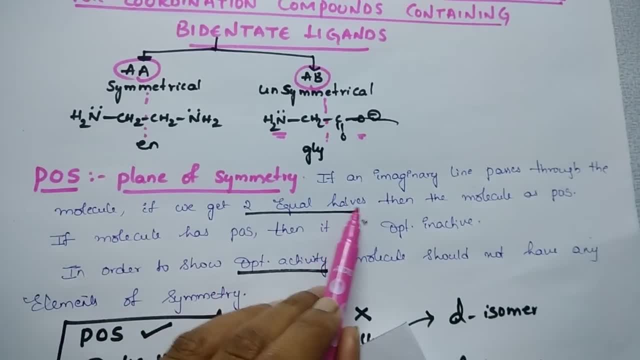 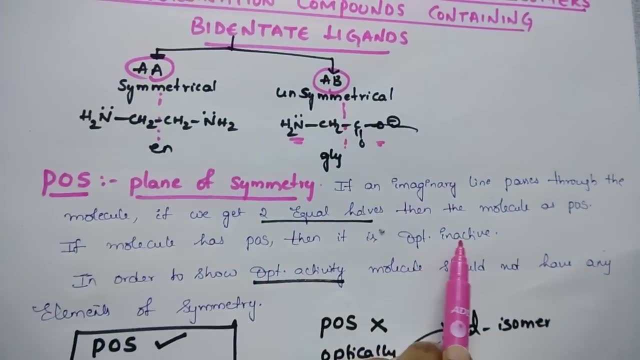 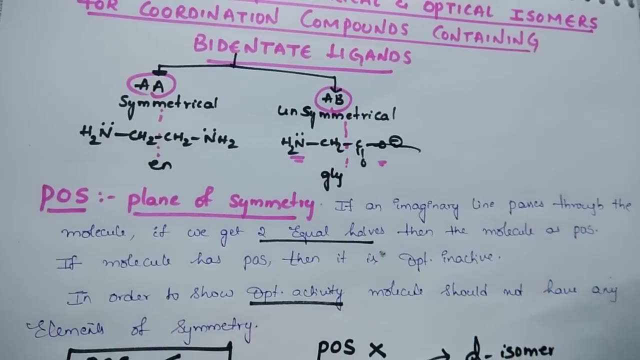 Passes through the molecule. if you get two equal halves, Then the molecule has plane of symmetry. if the molecule has plane of symmetry, Then it is optically inactive is a clear. if it is having plane of symmetry, Then it is optically inactive in order to show optical activity. 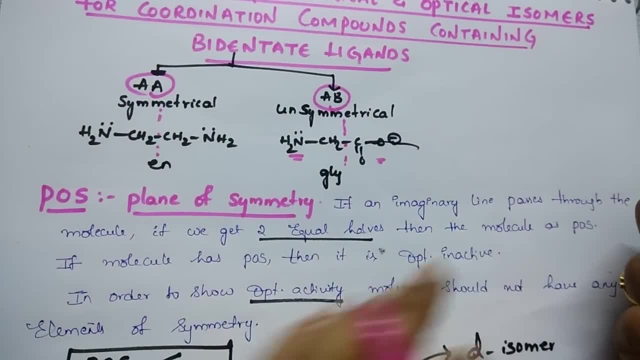 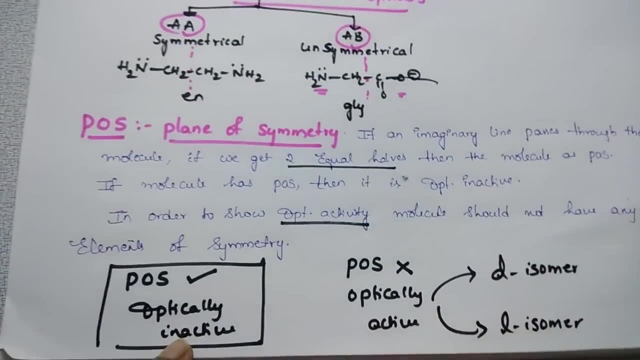 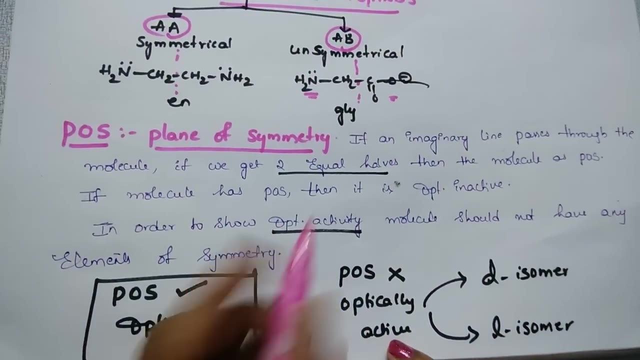 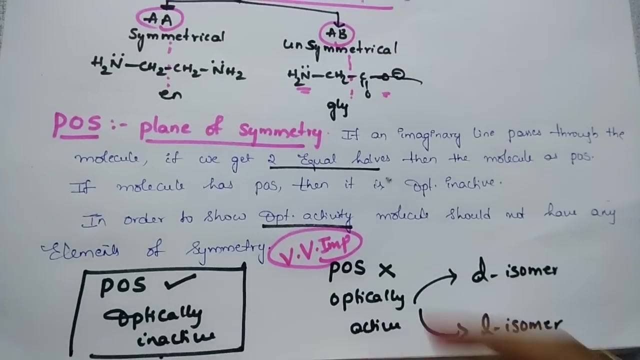 Molecules should not have any elements of symmetry. Suppose, if it is having plane of symmetry, students, that is optically inactive. very, very, very key point: If it is not having plane of symmetry, then it is optically active. Very, very important If it is optically active. 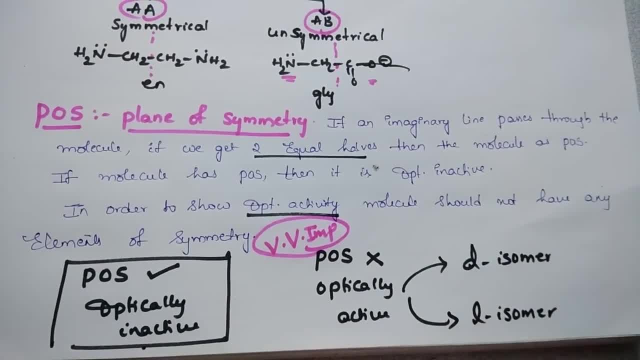 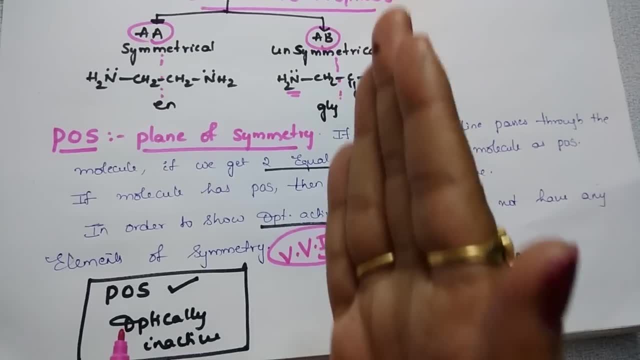 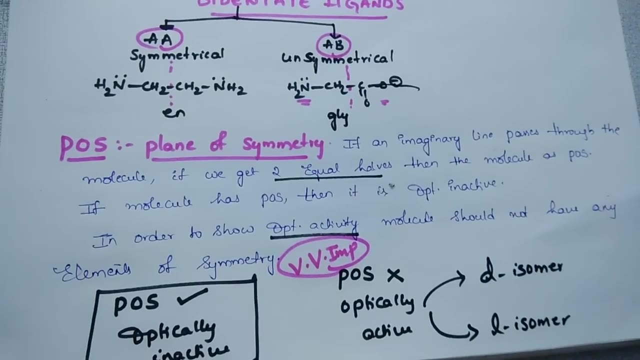 Then it is optically inactive. two isomers are possible to that optically active. one one is d isomer, another one is l isomer. what i am telling you, if you cut into two equal halves, means an imaginary line passes. if you get two equal halves, that is having plane of symmetry. to understand this better, i'll show you my sun. 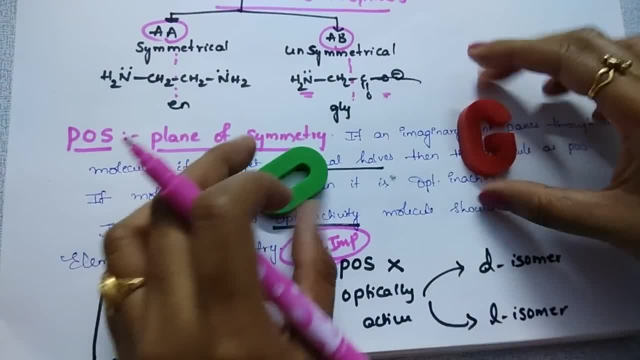 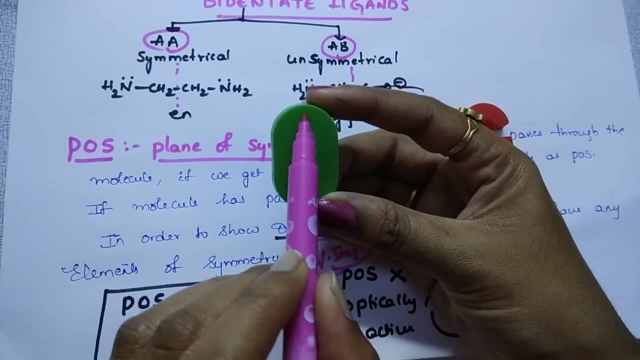 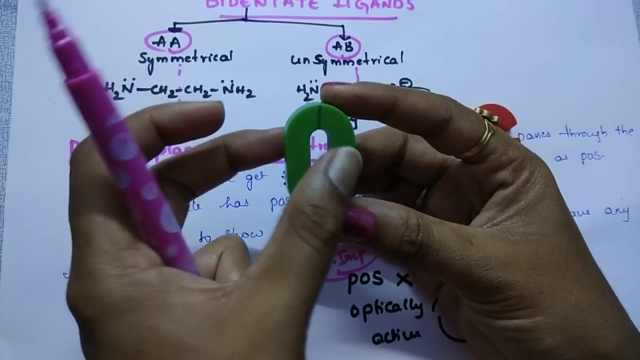 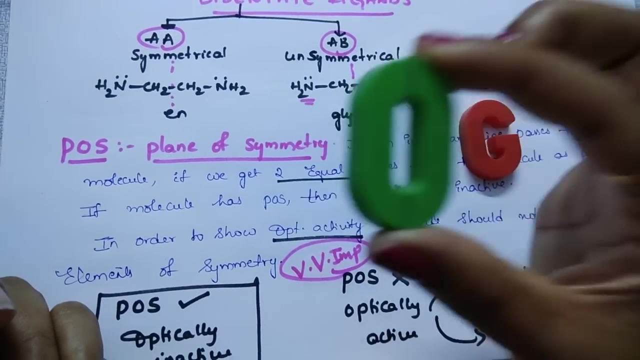 alphabets. see here: suppose this is the alphabet o. if the imaginary line passes like this, then we get two parts. this is one part and this side one part. right, both are same. then this is called: suppose. if it is an coordination compound, then it is optically inactive why it is having. 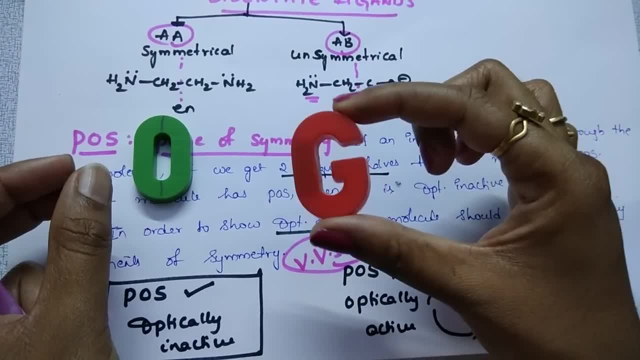 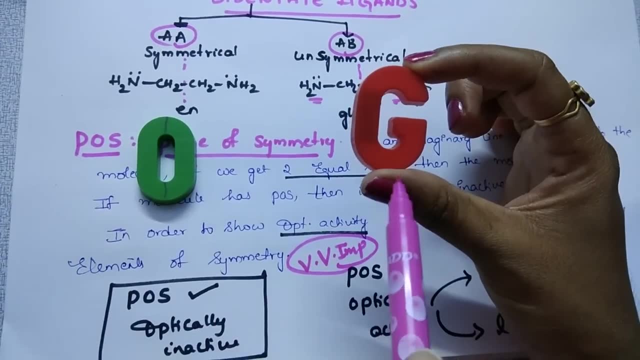 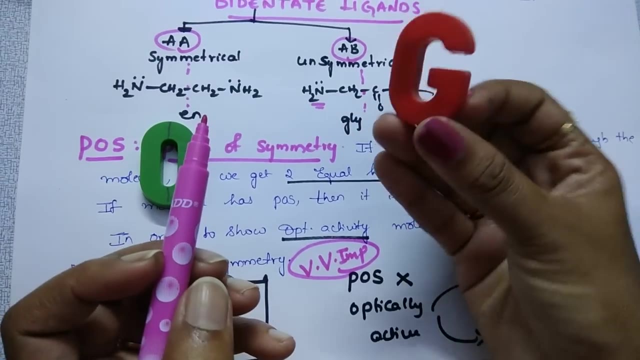 plane of symmetry. and see this alphabet, you can see that it is having plane of symmetry. and see this alphabet: d isomer. another one is g. if an imaginary line passes like this: no two equal halves. if it passes like this: no two equal halves. if passes like this: no two equal halves means this: suppose, if this g is an coordination. 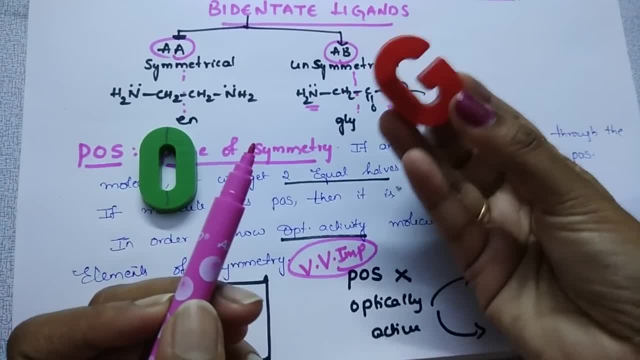 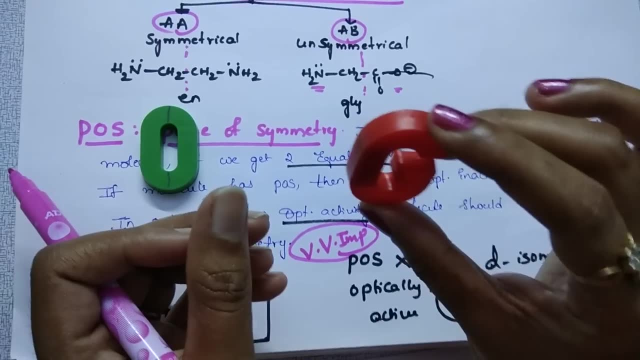 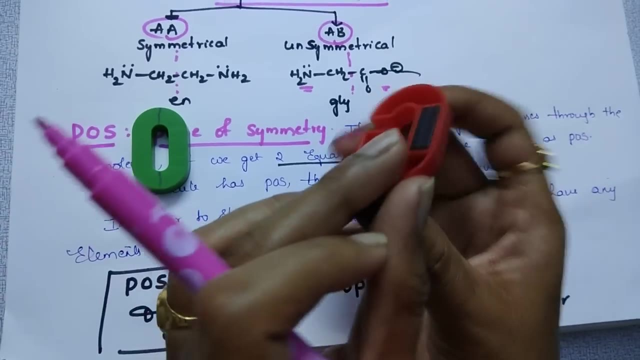 compound, then it is optically active. why? because it is not having plane of symmetry. if it is optically active, in this case, it can rotate the light either towards the right or either towards the left. if it is rotating either towards the right, we call it as d form. 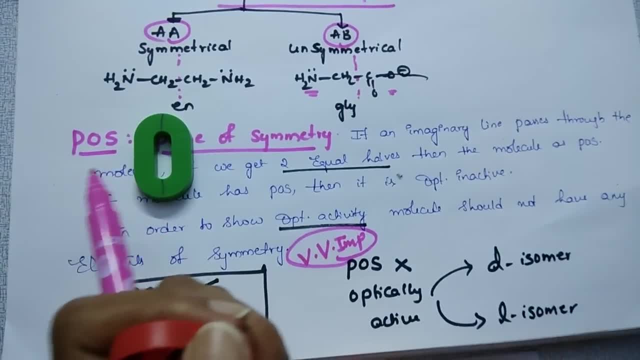 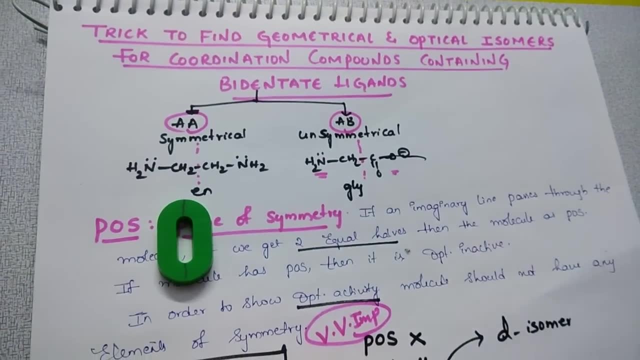 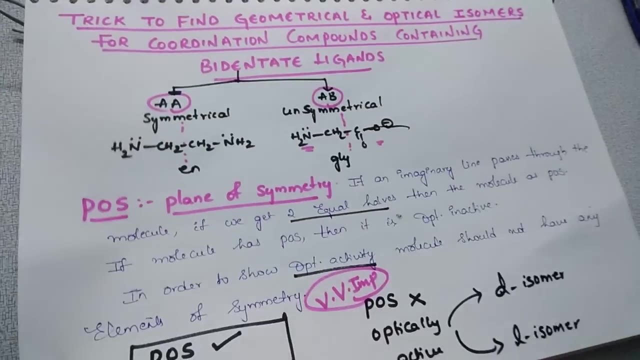 if it is rotating towards the left, then we call it as l form is a clear. now let's start our session with different examples. please watch up to the end of the video. really it, it is going to be amazing. it will be helpful for you see this complex m a a thrice means this is an imaginary line. 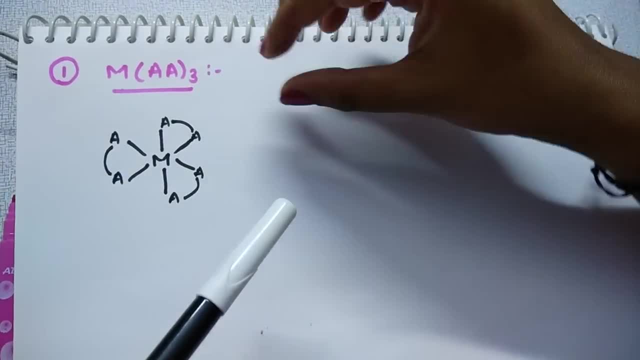 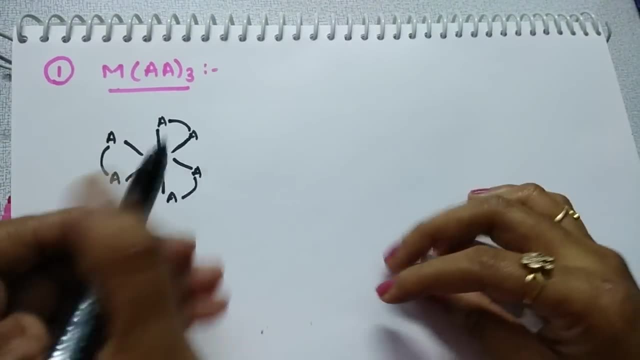 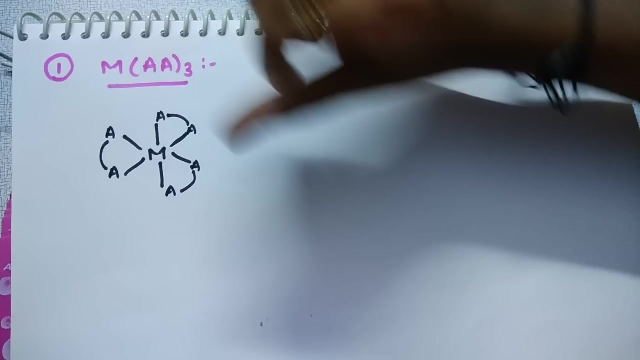 this is a is bidentate ligands. it is there three bidentate ligands are there right. and this is the complex in this complex. if you see, if i rotate these two means, if i interchange these two positions, again i get the same structure. if i do this, if i interchange this, i get the same. 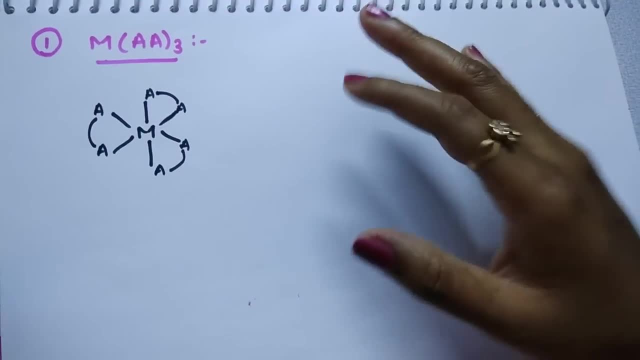 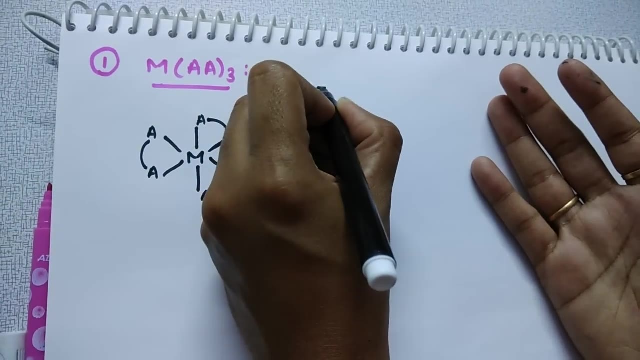 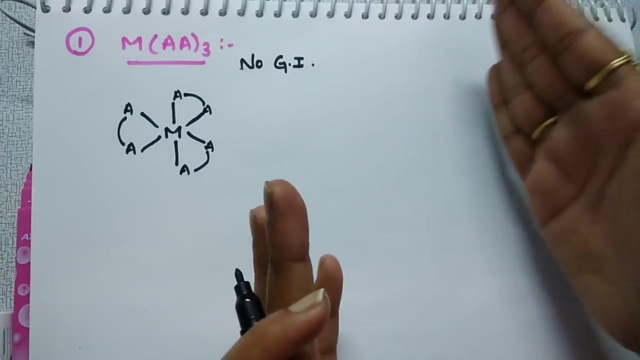 structure. if i interchange this i get the same structure. means here there is no geometrical summarism. means no other combinations is possible. no gi to this structure. now coming to the optical activity. whether it shows optical activity or not it completely depends upon plane of symmetry pos. 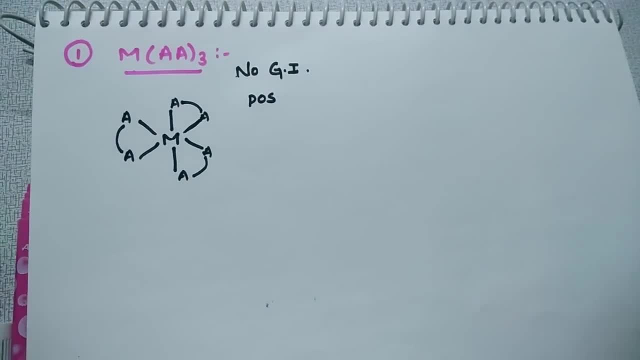 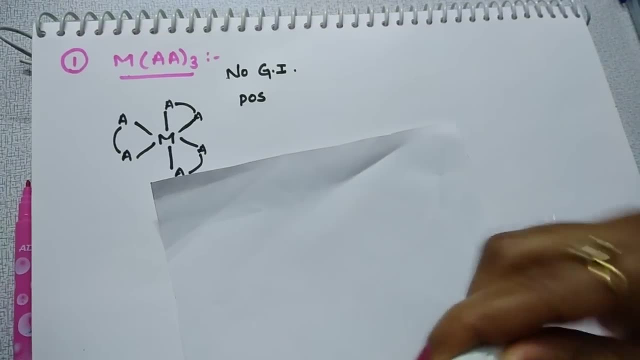 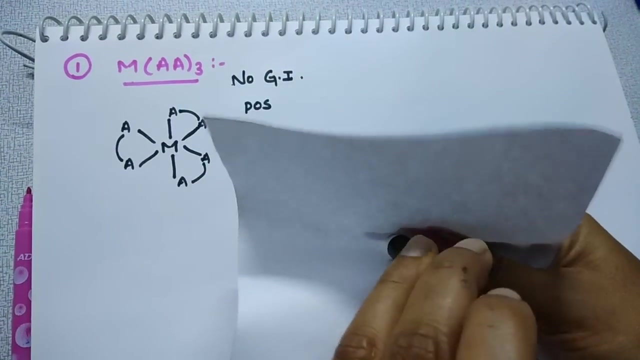 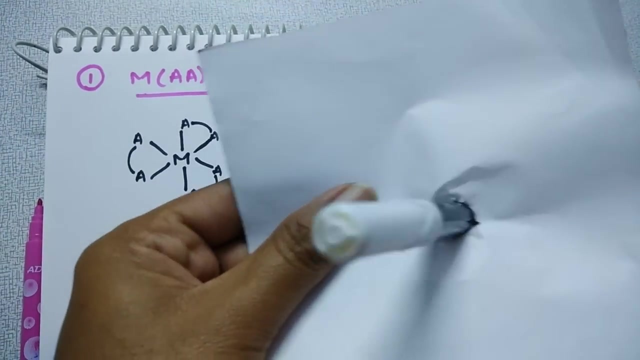 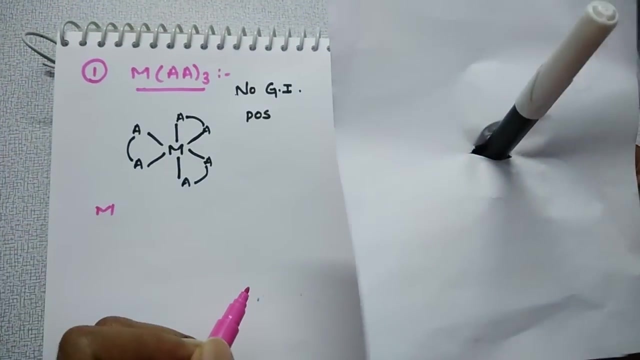 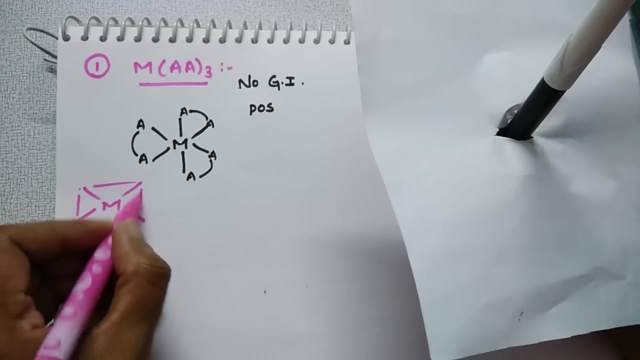 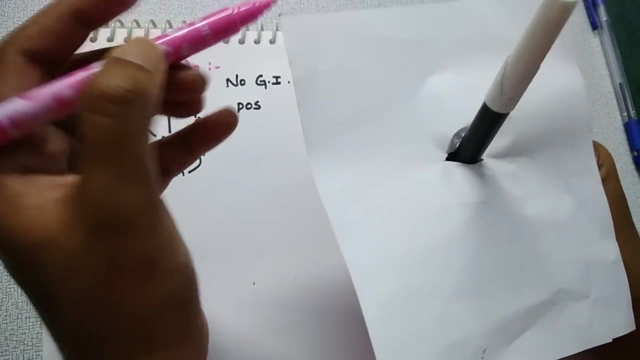 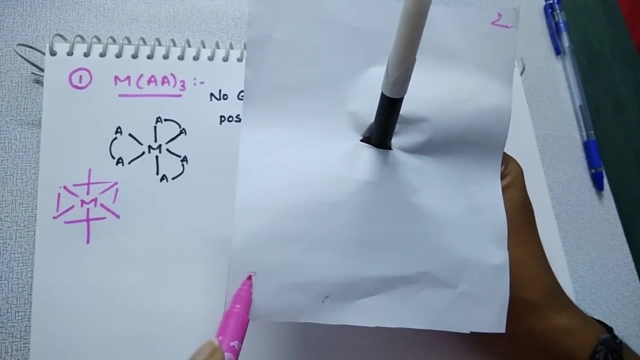 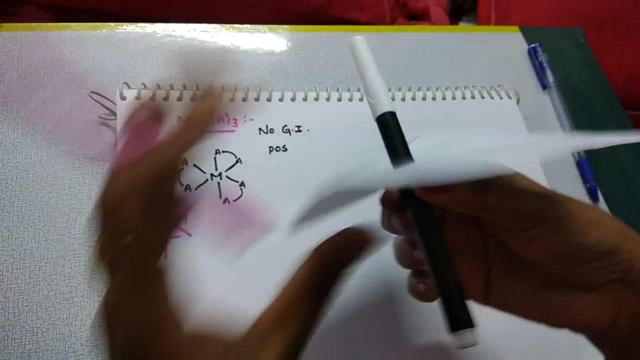 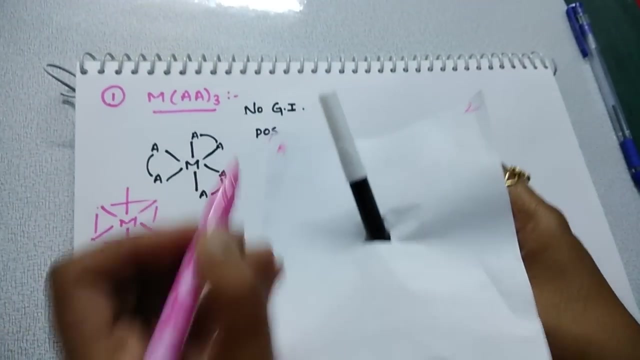 is a clear students to understand this very, very important thing i am going to discuss now. see here, this is the four corners: one, two, three, four. one is above the plane, other one is below the plane. clear now, this is a bidentate ligand. so here a, here a bidentate. that too symmetrical. 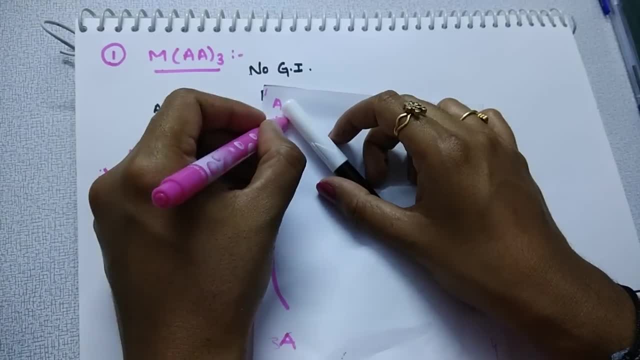 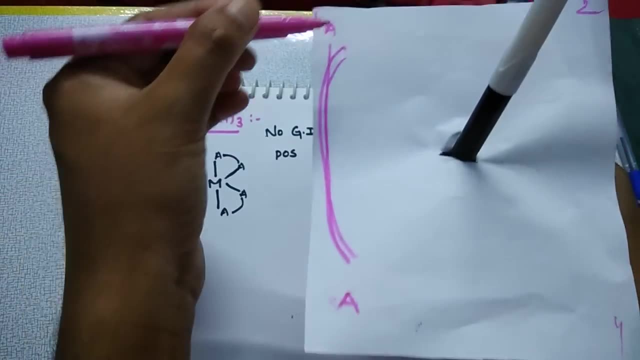 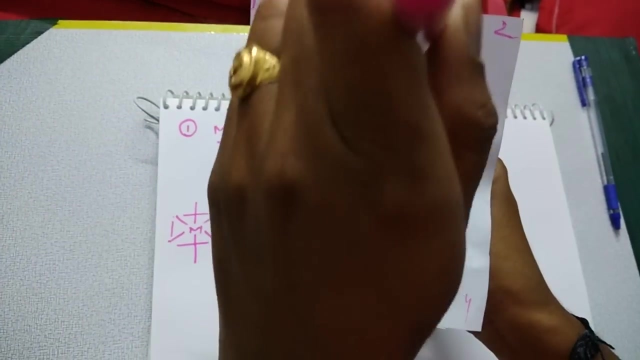 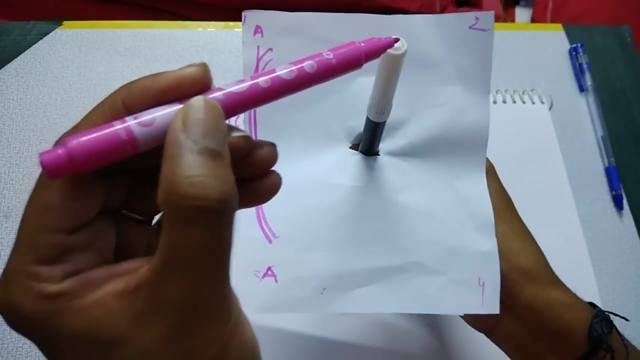 this is the ring. okay, like this, one ligand is present, bidentate ligand, and here one side right. please try to understand this very, very important to understand optical activity and this ligand here, one a, and it coordinates with this. like this you're following. 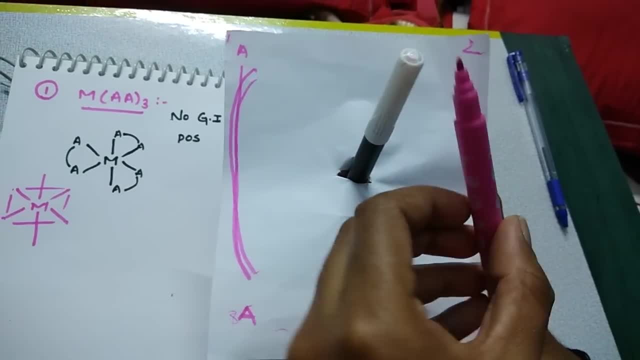 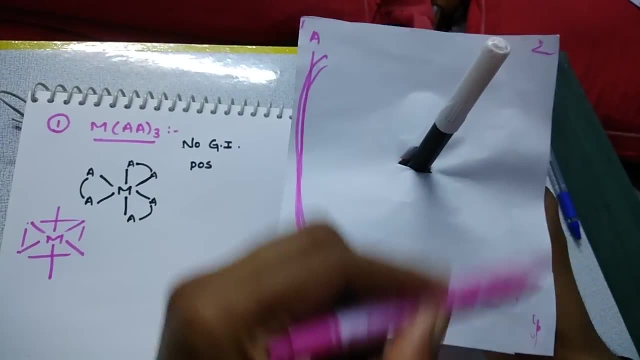 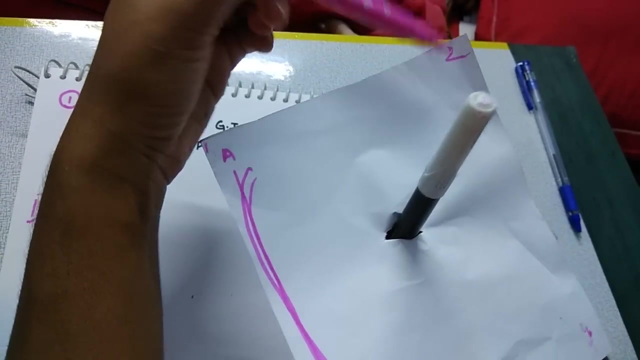 here like this: one ligand is present, bidentate like end here a here, hey, hey, Harry, you understand this right. like this means like this on the one plane and like this on one plane and this second position and it down one more leg. and is there no students see here like this: 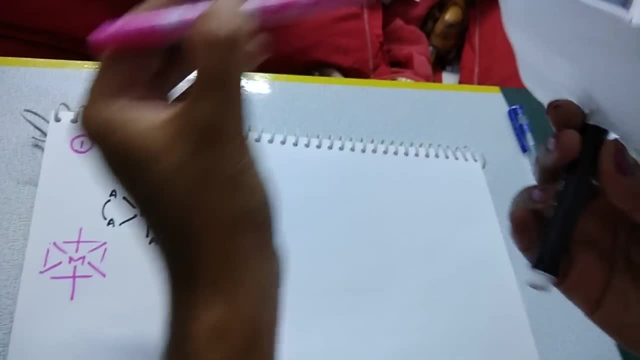 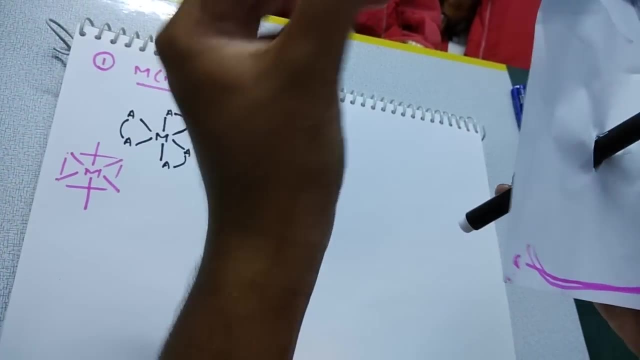 second position. second position and like this means here one by detail again. and the third position: here flow, here the bidented position. this bidentate position means like this: here oneแลòs And here like this one ligand and this side and here one more. 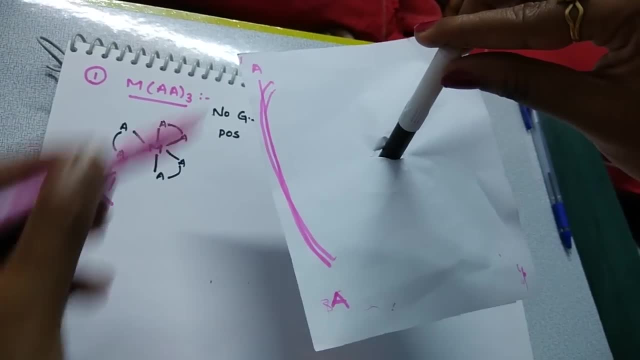 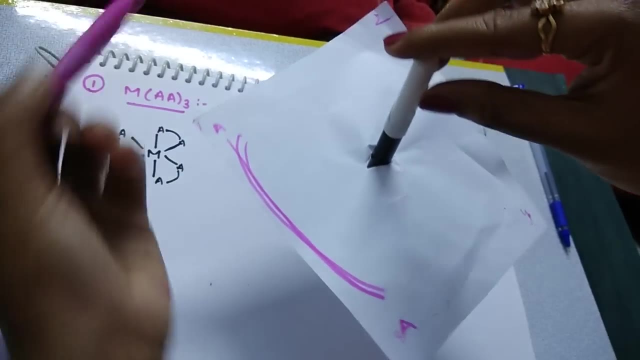 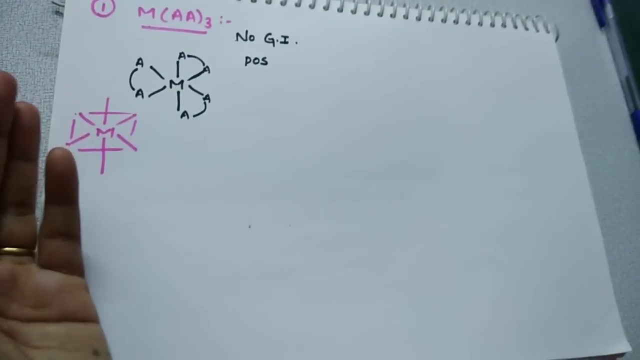 Got it. See, Like this one, Like this one And down. like this one Means what I want to tell you is 3 bidentate ligands are in different planes. 3 are in different planes, So you cannot cut that into 2 equal halves. 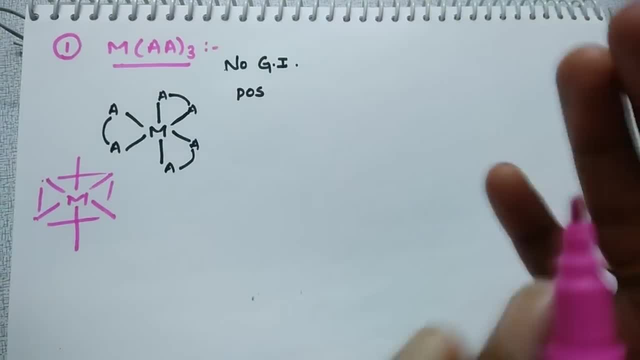 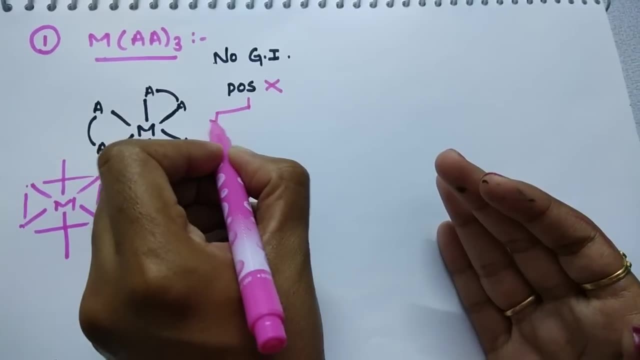 Please try to understand. 3 are different planes. You cannot cut into 2. equal halves Means it is not having plane of symmetry. If it is not having plane of symmetry, then how many isomers are possible? 2 isomers because it is optically active. 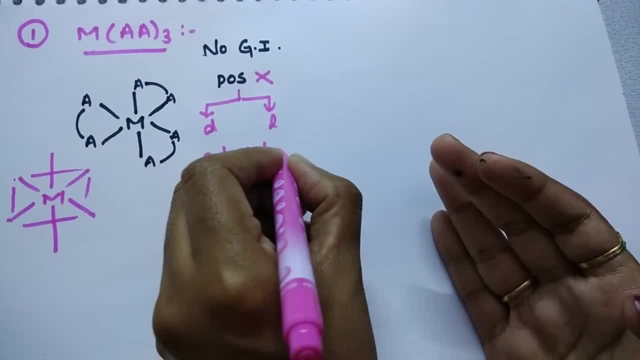 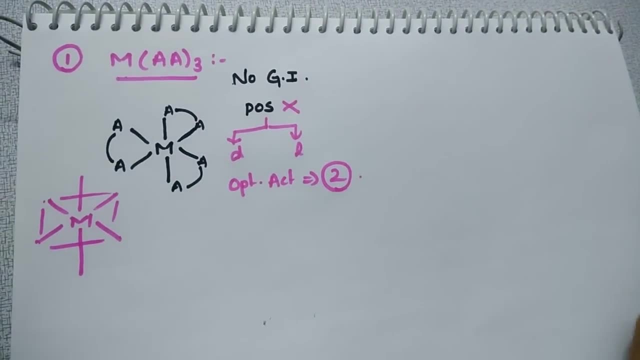 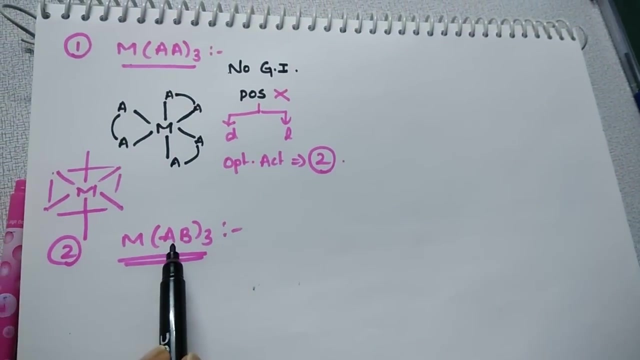 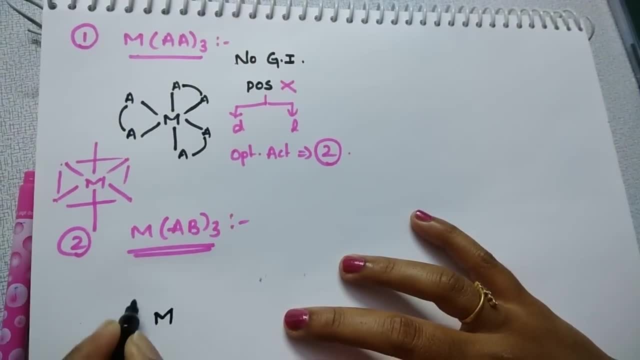 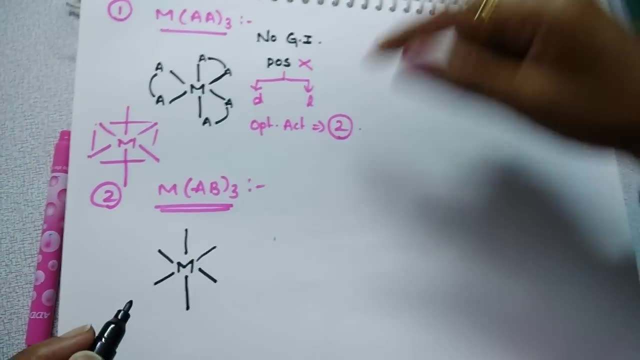 M, ab3, ab3.. Unsymmetrical ligands: 3 are present. See here These 4 on the plane. This is above the plane. This is below the plane. Here I am representing the 3D structure into 2D. 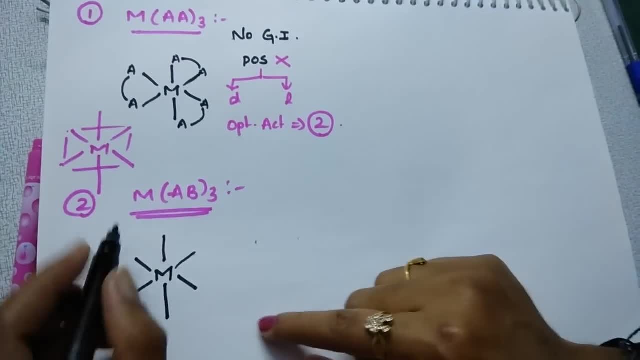 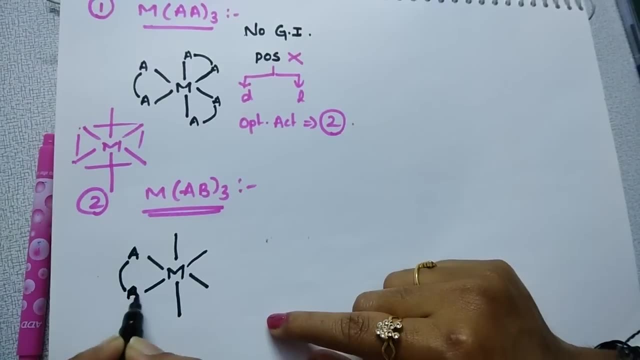 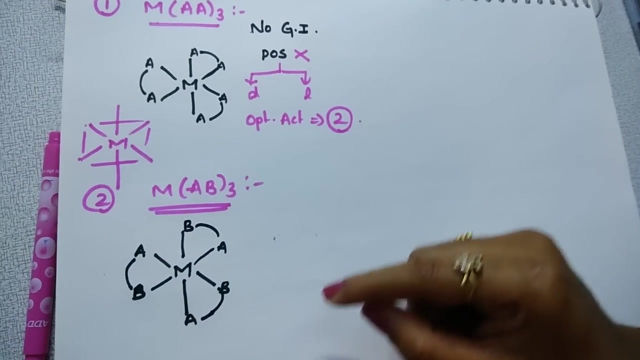 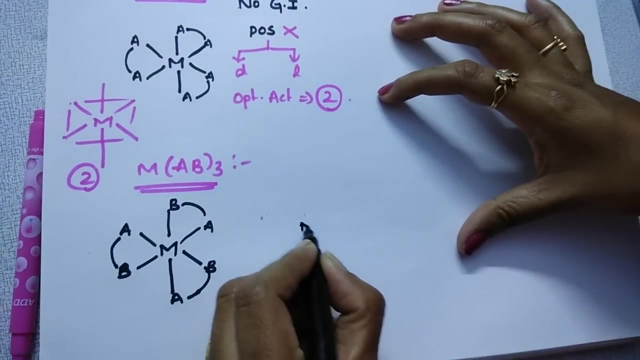 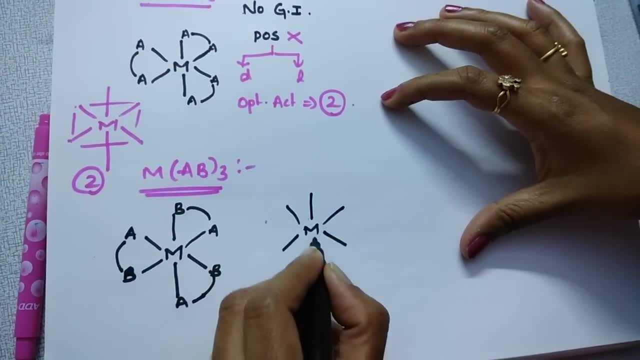 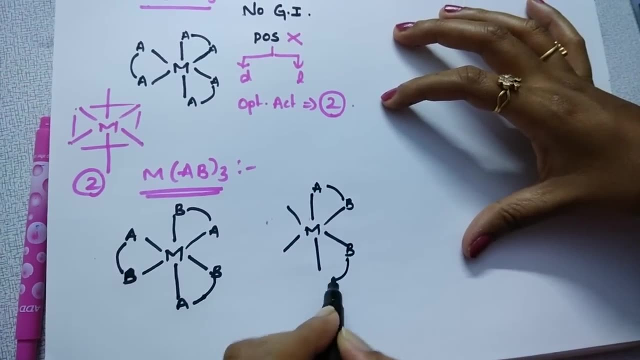 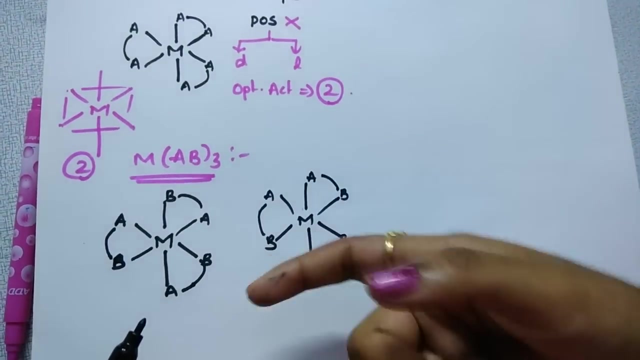 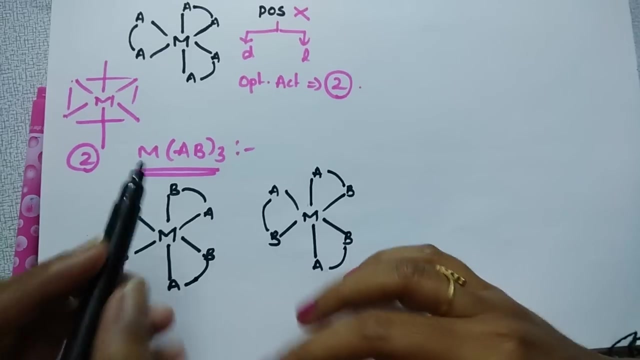 here. if I interchange these two, then I get here A, here B. remaining everything will be same. if I interchange any other two, I will get the same structure. just you try it. if you interchange again anything, you get the same structure. how to identify that? you get the same structure or not. just you see the opposite things here, B and A, one combination. 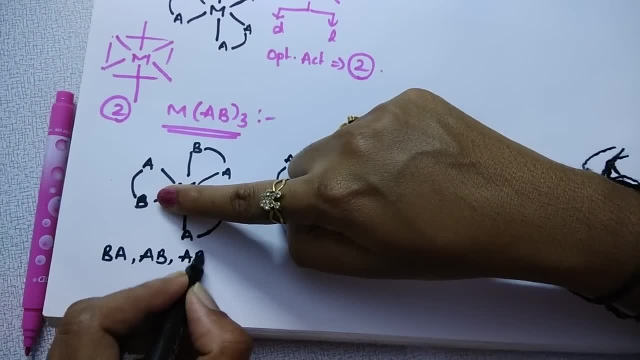 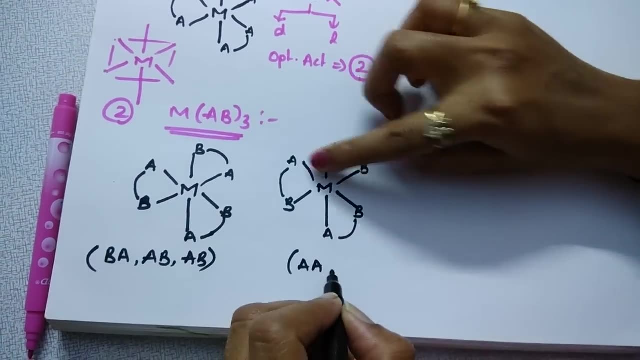 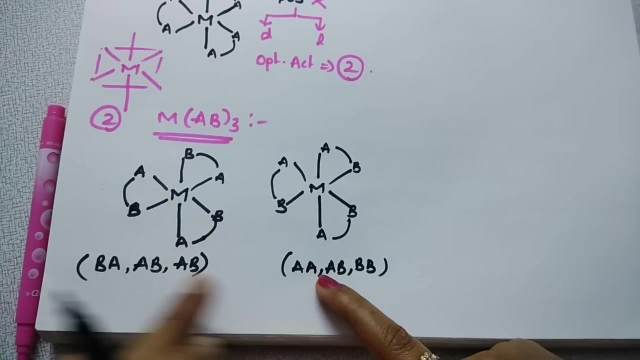 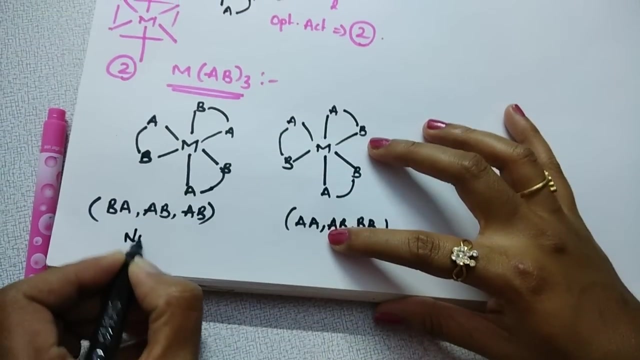 AB is one combination and AB is one more combination and in this case AA, AA one combination, AB one combination, BB one combination. See here: AA is there, here one, AA is not there. both are different combination. so the number of possible geometrical isomers are: how many students? number of geometrical isomers are. 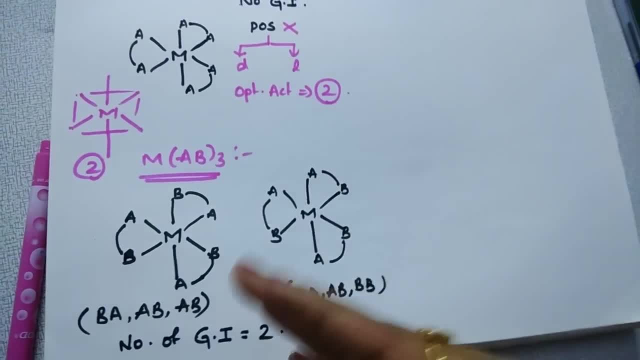 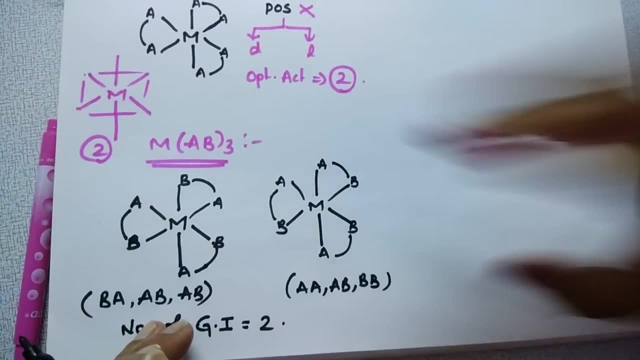 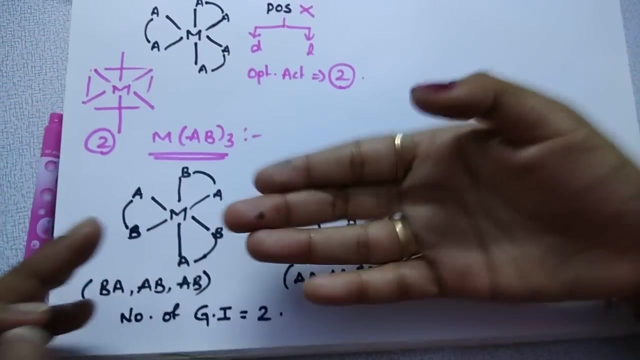 two and one more thing: to find the optical activity just now I discussed. if you see this molecule and if you feel I will cut like this I get two equal or no, it's wrong. This is in imagine. in 3D structure, this bidental ligands three are present in three different 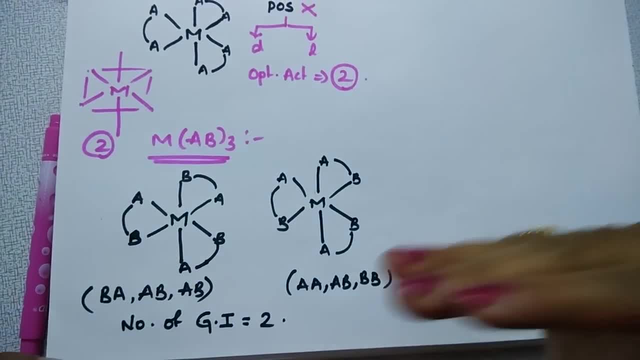 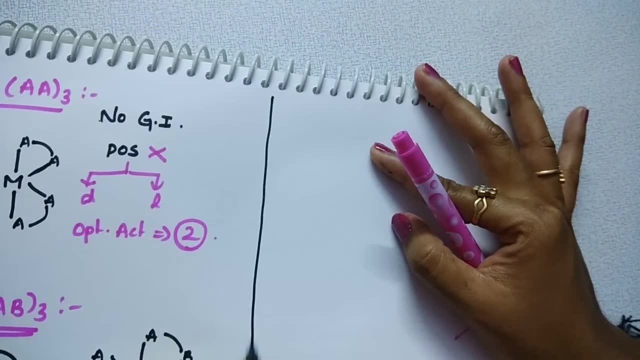 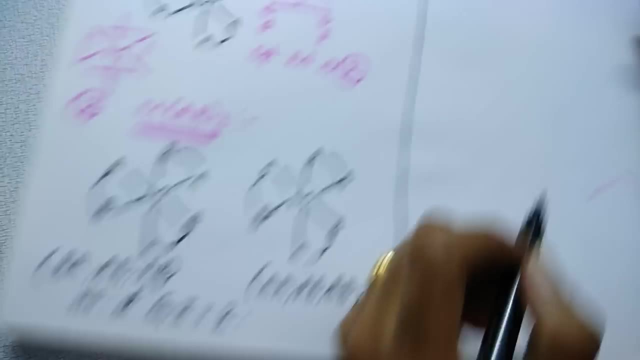 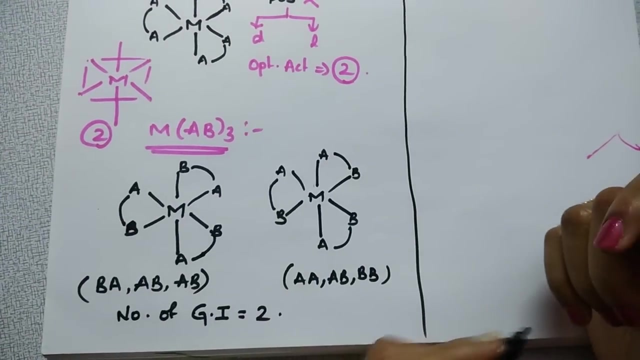 planes you cannot cut into two equal halves, then it shows that it is what it is: optically active, if it is optically active. optically active, how many isomers are possible? how many? two, four, three, three options. I am giving two, three, four. what is your answer? it gives D. 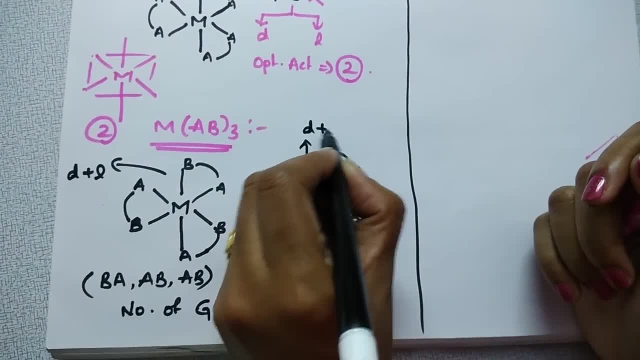 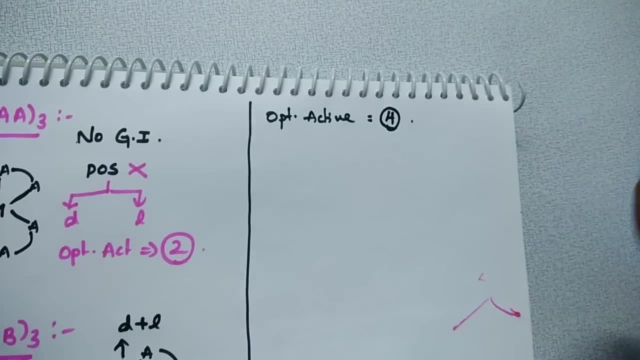 and L forms. It gives D and L forms. It gives D and L forms. It gives D and L form. It gives D and L form. Total: here two, here two: total optically active isomers are four. let us see one more example. 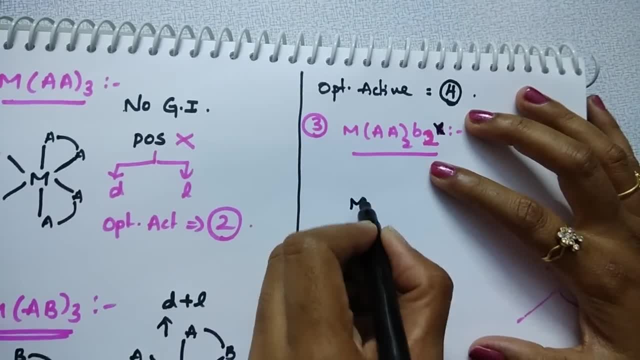 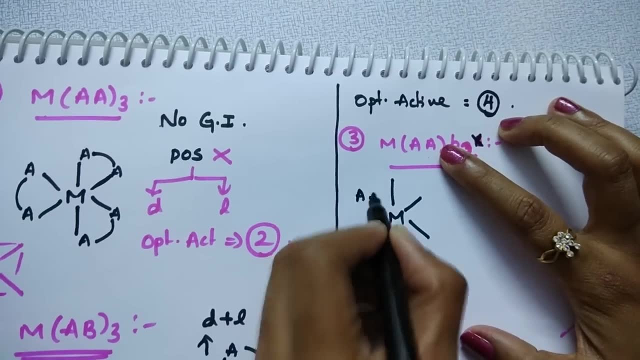 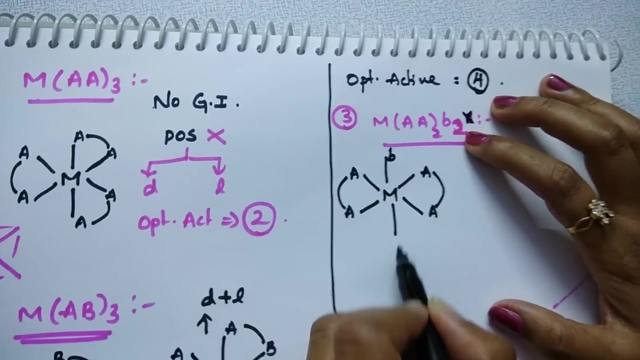 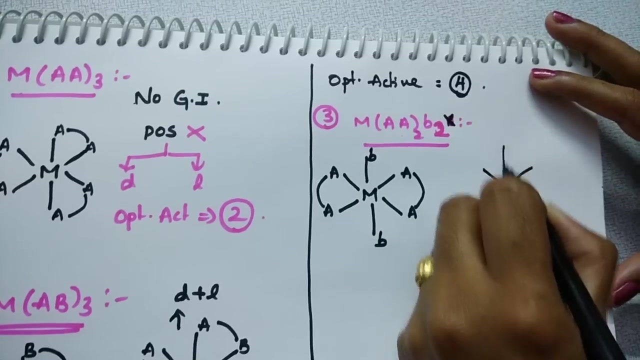 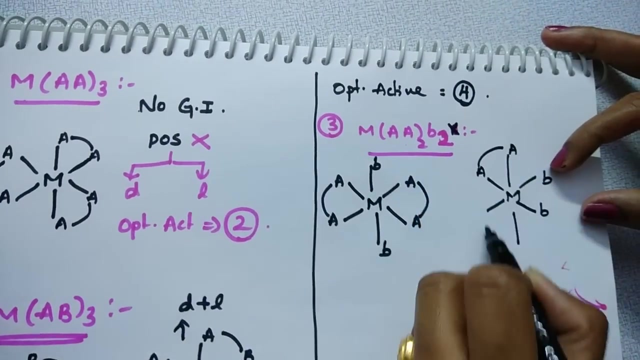 M, A, A twice Btwo: first, draw the geometrical isomers. two symmetrical bidential ligands are there. right, I will write like this: and two monodentate ligands are there. ok, okay, one combination. two B's are side by side. yes, any other combination is possible. 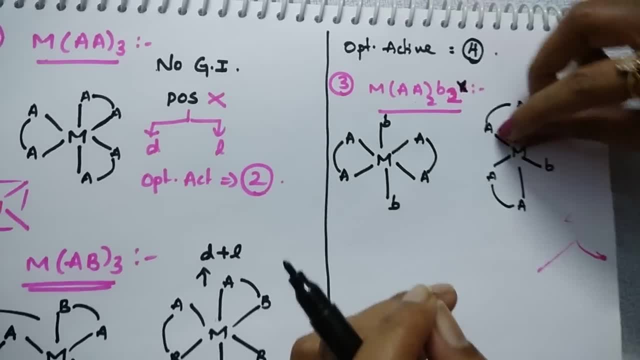 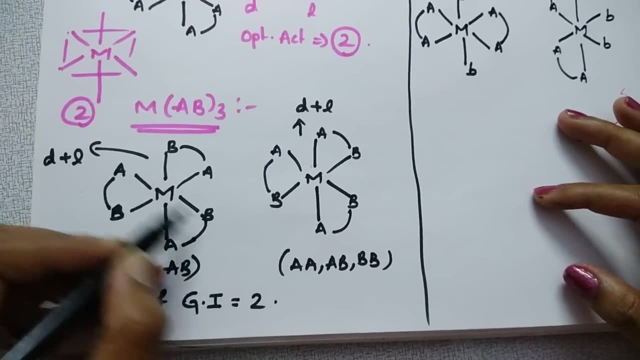 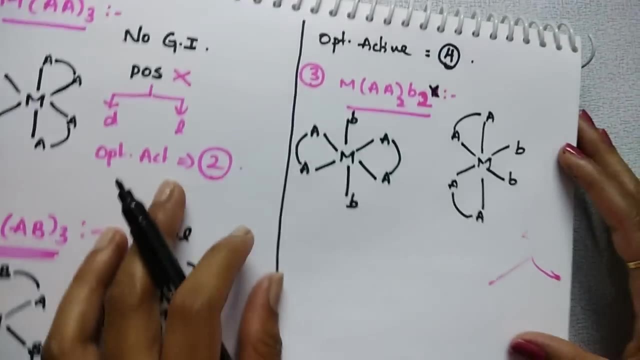 no, only these two are possible. you just try it. if you try also, you get the same kind of structures. how to identify? I told you know what are the groups opposite to each other. you just write and see. then you will come to know whether both are same or not. 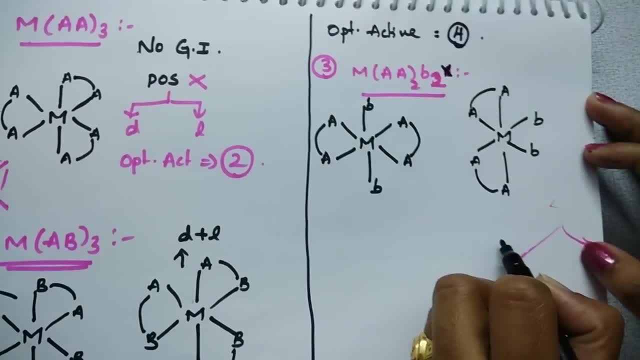 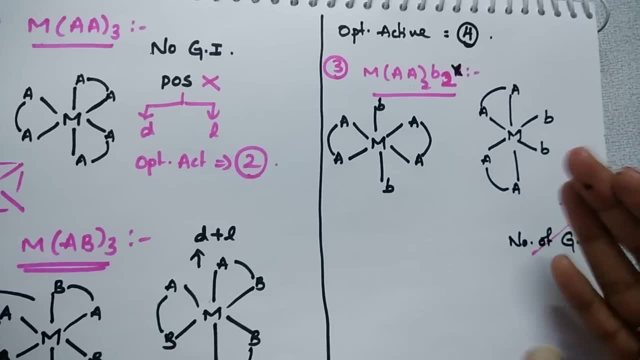 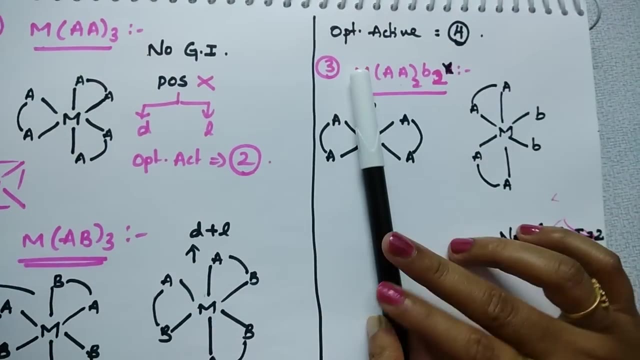 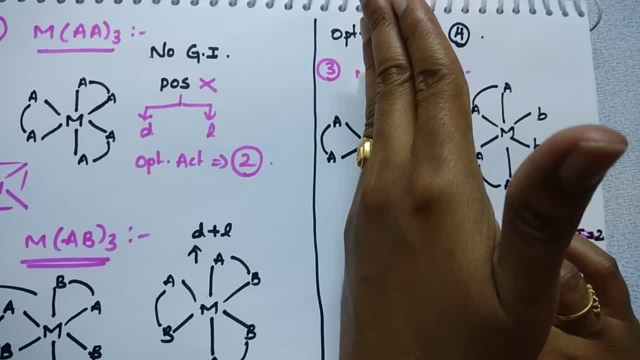 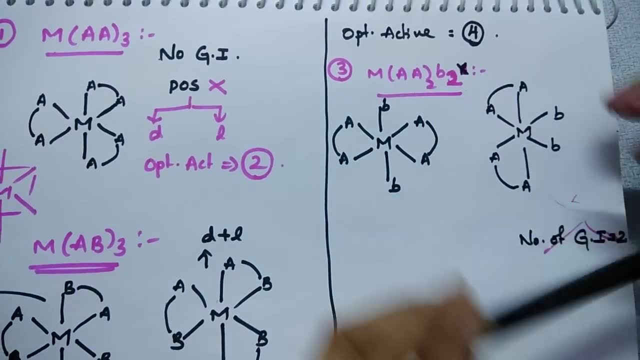 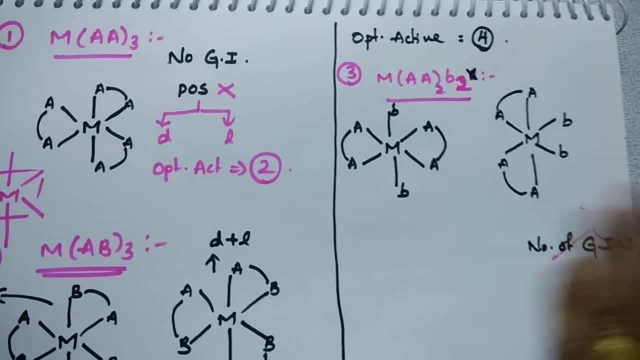 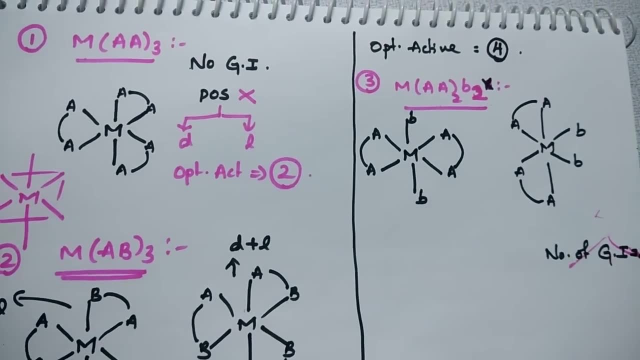 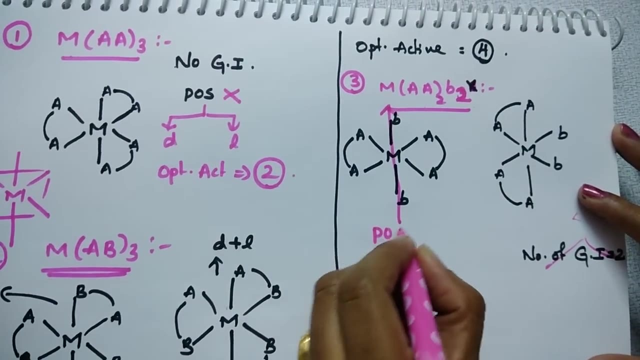 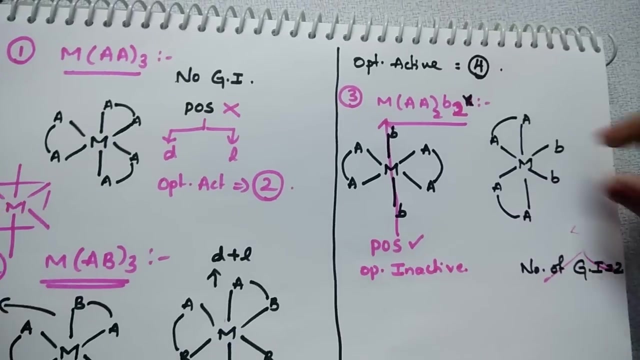 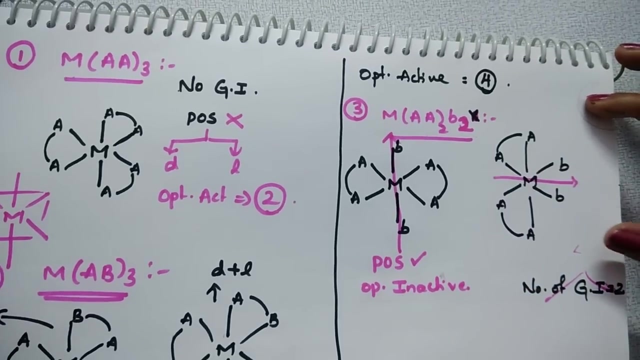 get two equal halves. yes, then you will be wrong. see, cut the molecule like this, two equal halves you get then it is having plane of symmetry and optically inactive and this cis form, if you see, transform is optically inactive and cis form, if you see, you cannot cut the molecule like this. i already discussed with you. these two are not in the same. 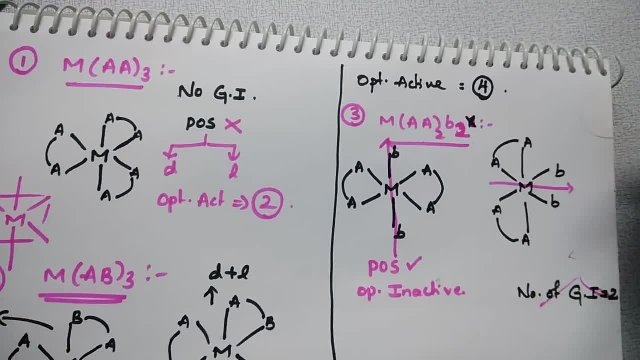 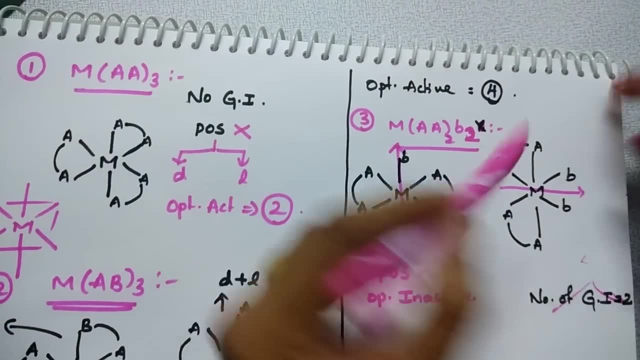 plane. if you see this 2d structure, it is not in the same plane. it is not in the same plane and you cut it. it is wrong. it is present in the three-dimensional structure. this is one plane and this is in another plane. it is not having plane of symmetry and this is optically. 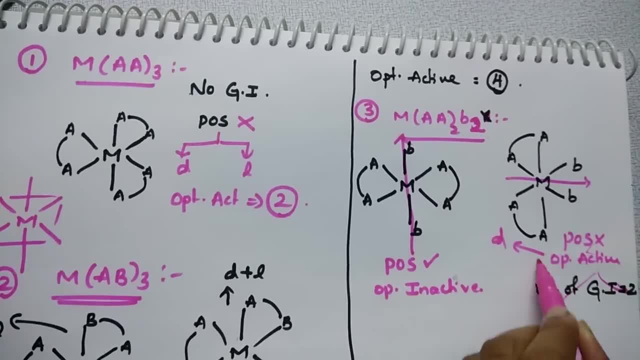 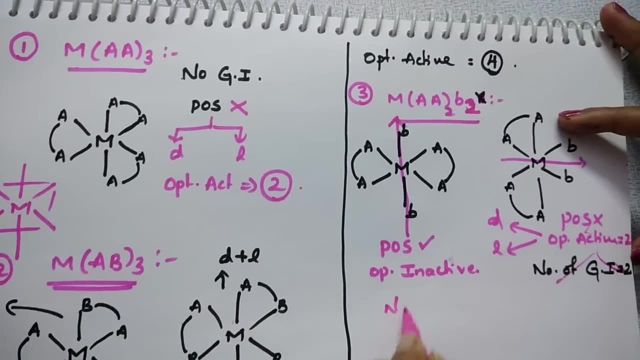 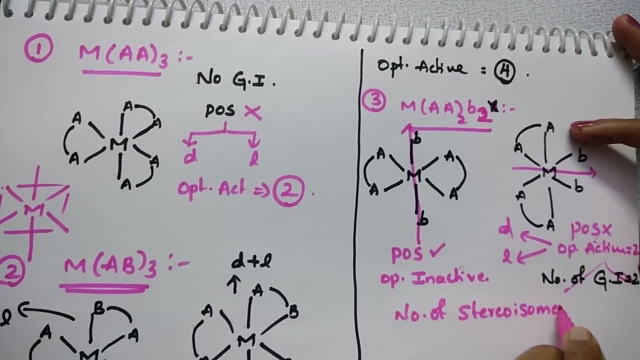 active if it is optically active. d form is possible, l form is possible. so total optically active isomers are two and number of stereoisomers are how many students? number of stereoisomers means both optically inactive forms and optically active forms. how many are? 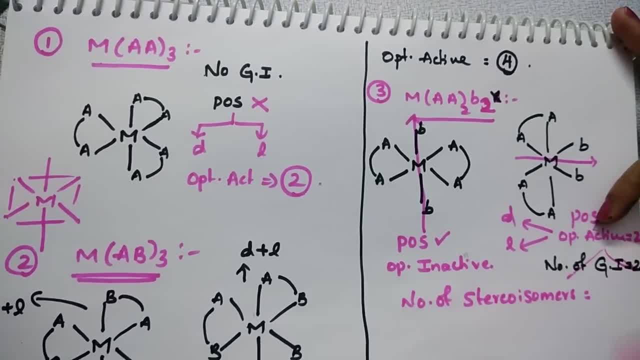 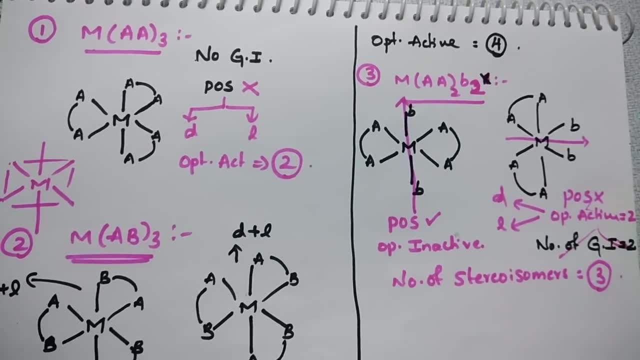 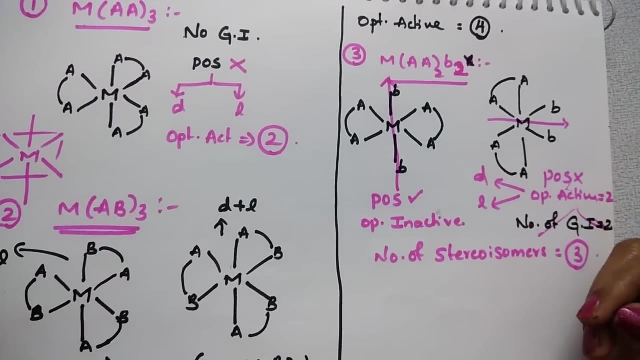 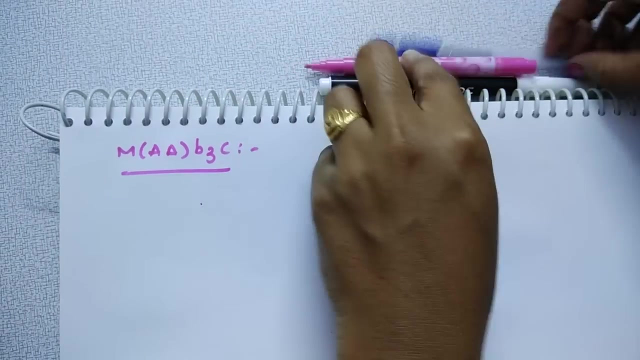 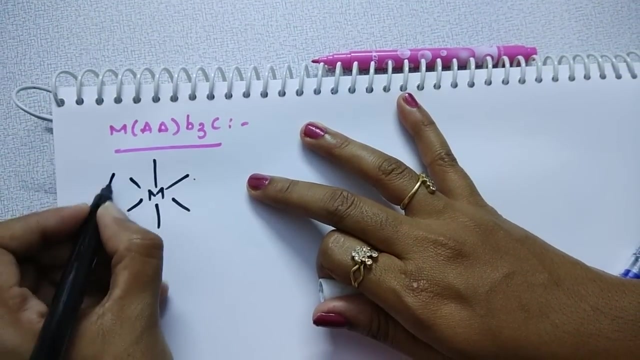 possible. two plus one, total three are possible. number of stereoisomers: how many three stereoisomers are possible? and now I am going to tell you an excellent trick. this trick will be useful for you. see this. first, find number of geometrical isomers. write the different possible structures a here, BB. 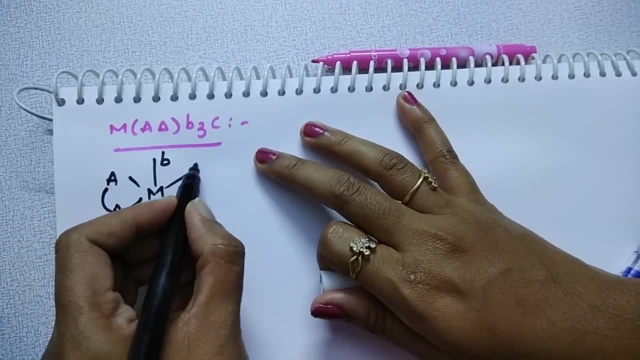 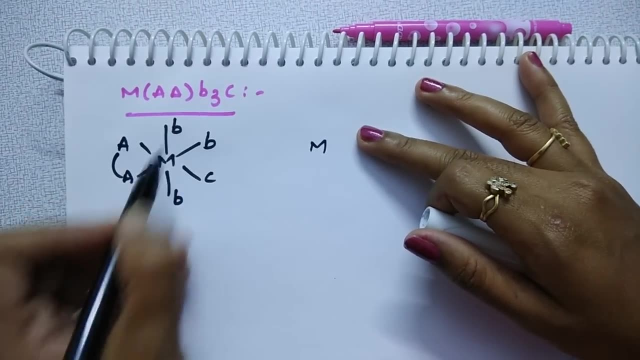 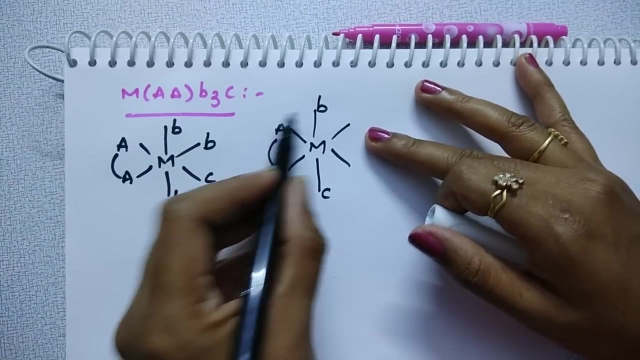 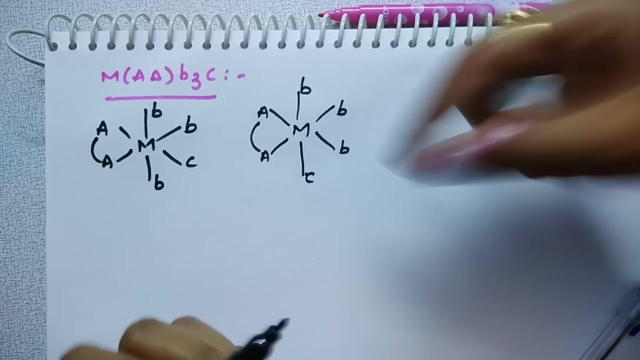 B, 3 C. no, I'll take BB- opposite side- and BC. any other isomer is possible. I'll take opposite: 1 B, 1 C, B, C. so what is left? BB, BC is left right. any other combination is possible, you try it. you, these only two. 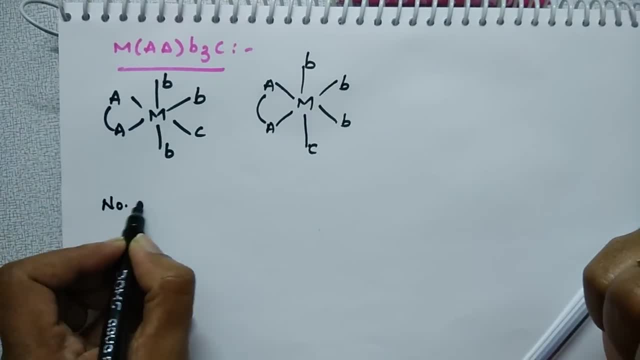 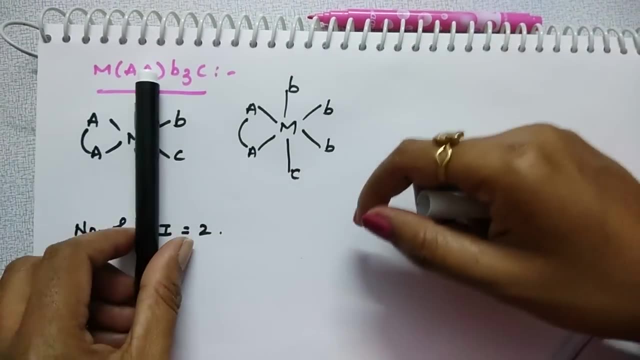 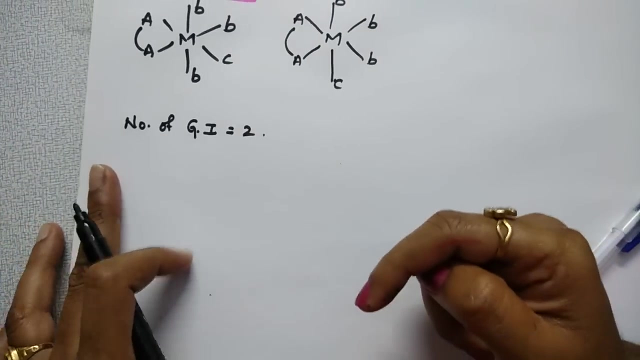 are possible. so number of geometrical isomers are two. and coming to the optical activity, how to find if you cut into equal halves and all these things. it takes some time for you. so I am, I am going to tell you an excellent trick. that suppose, if two opposite groups are same, if two opposite groups are. 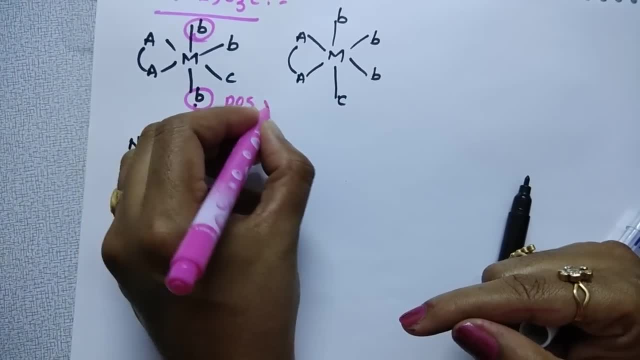 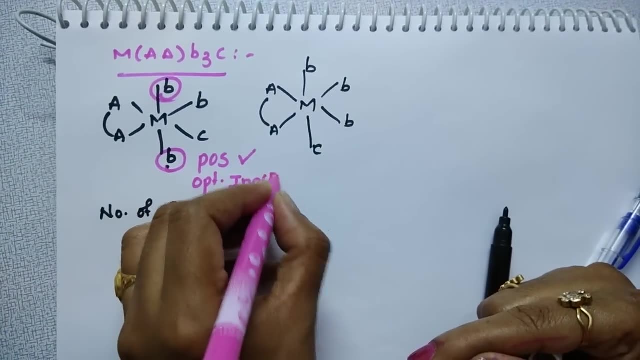 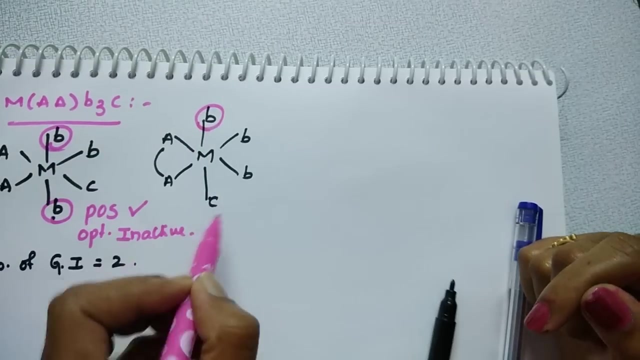 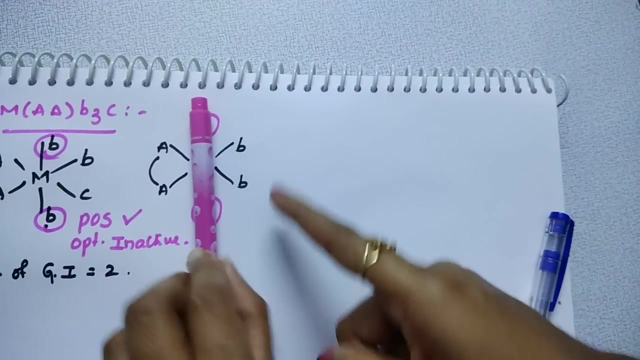 same, then it is having plane of symmetry. if it is having plane of symmetry, then optically inactive, fine. when two opposite groups are same. if supposed two opposite groups are different like same, if supposed two opposite groups are different like this, then you should see the groups which are next to it side to it, decide side groups. if both groups are equal yourself, then you should run. you're very good and helpful to others, so put it in your stopping order: Lewis. to it side side groups: if both are equal have total 1990. to the opposite group: if both the groups are one, then you're good at 젤�ن. so if one of us decreses their mites then they'll have precisely the opposite group side group it will group if this is different. so depend on the way it's lived from this step, the groups which are next to it side to it, the opposite group. you have to be very good. 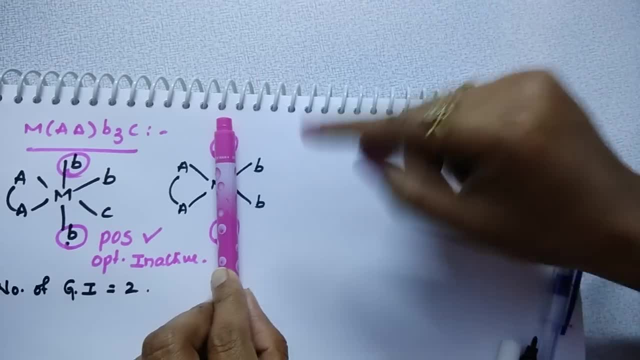 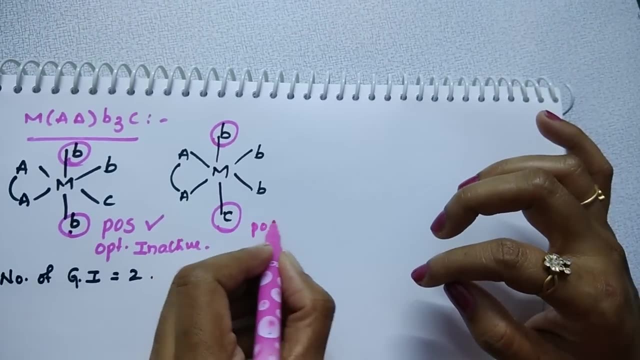 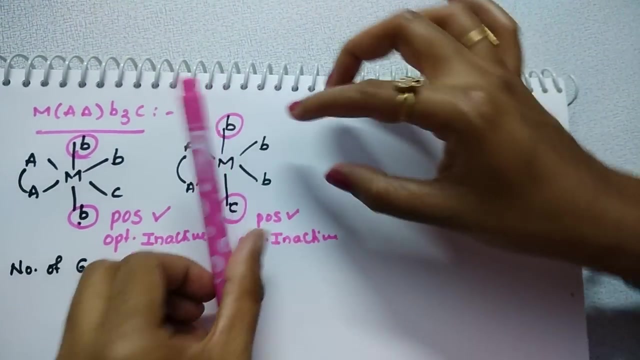 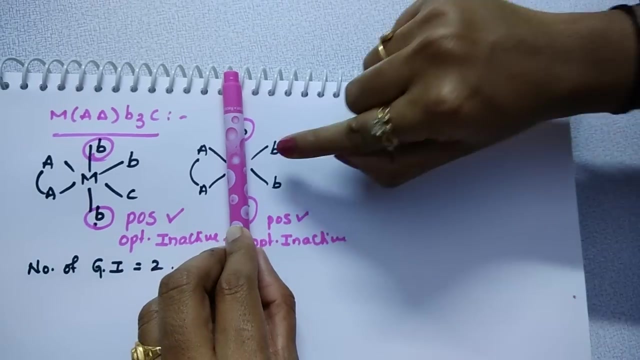 side groups. if both are same, AA, here ligands are same, like BB, then it is also having plane of symmetry. then it is also optically inactive, Suppose both the groups are different. if both the groups are different, then here also AA is there right, this side, suppose BC is there. 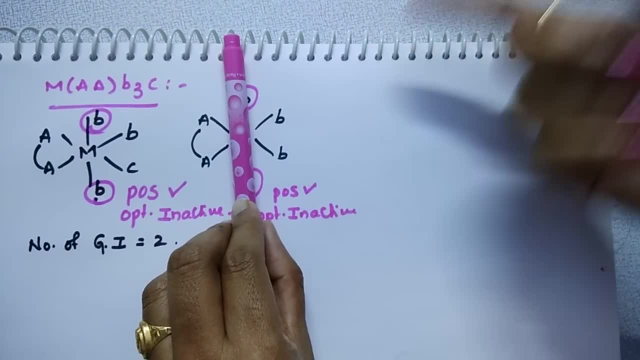 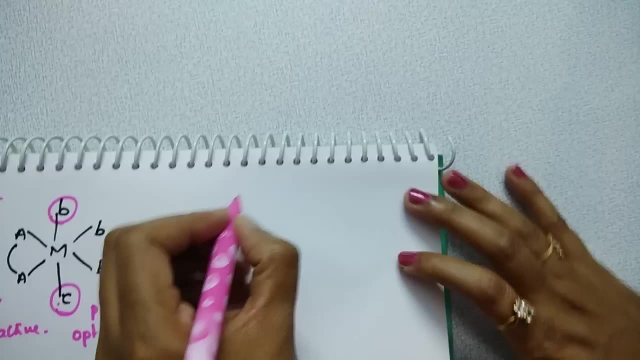 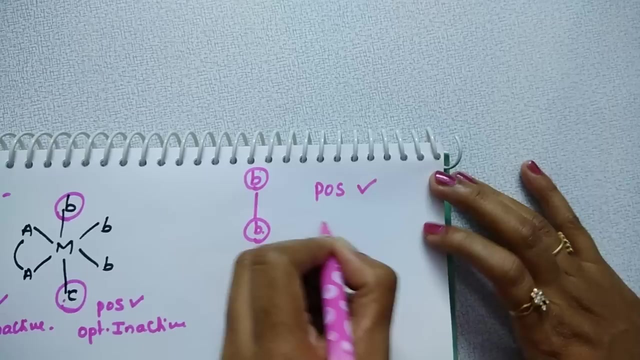 means both are different. then in that case that is not having plane of symmetry. that particular molecule is optically active. What is the trick? both the groups are BB, suppose same groups, then it is having plane of symmetry and optically inactive If opposite groups are. 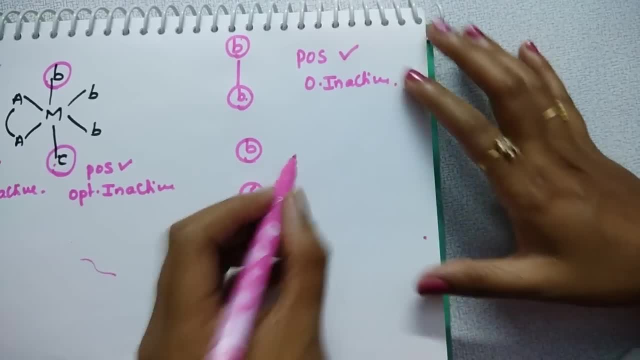 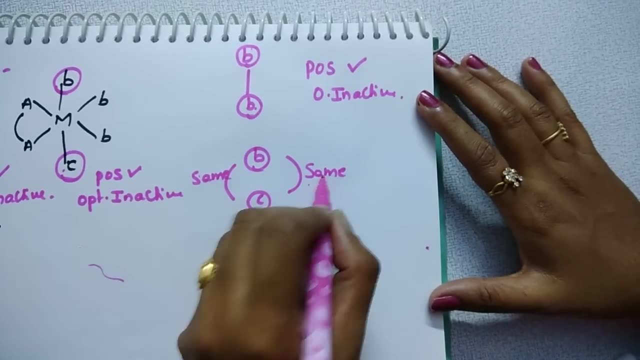 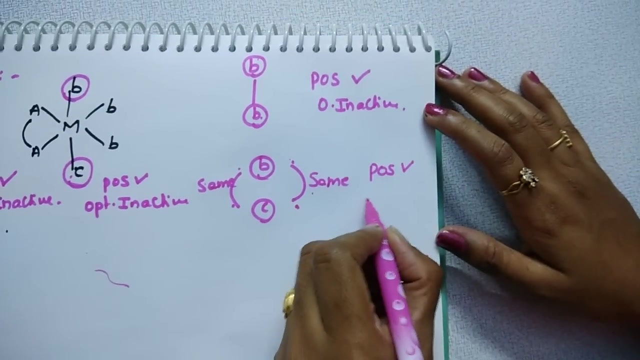 same, sorry, different, like BC, and you should see the next two groups are AA, Side groups are should be same. if side groups are same here and here ligands are same, then it is also having plane of symmetry and optically inactive. This is an excellent, very, very important. 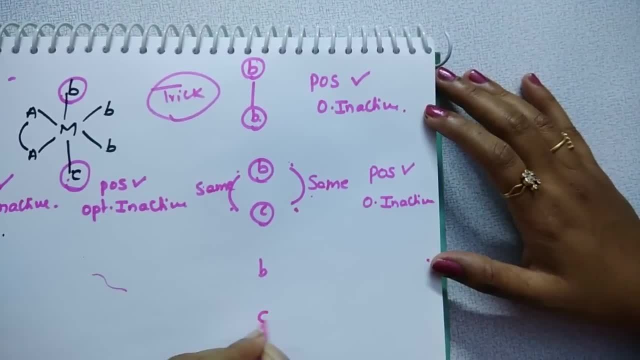 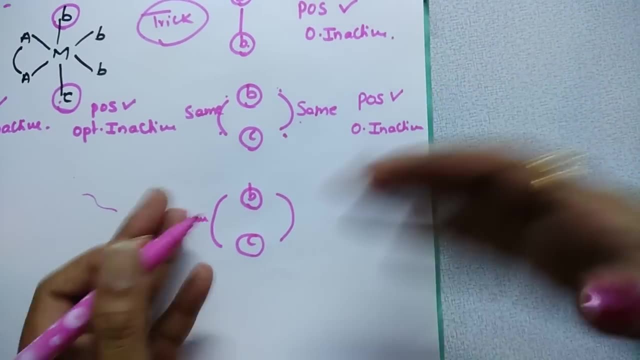 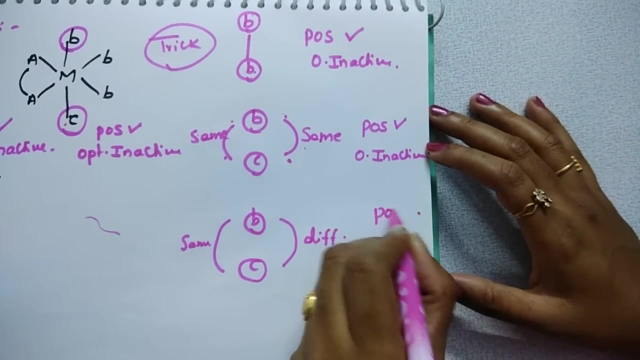 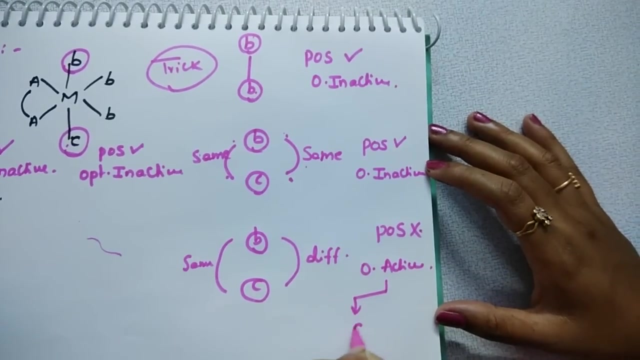 and if opposite groups are different, and you should see, this may be same, any one suppose one if same also, or both different also, For any one different, also different also. it is not having plane of symmetry, and that is optically active. if it is optically active, two forms are possible. one is D form and other one is L form. 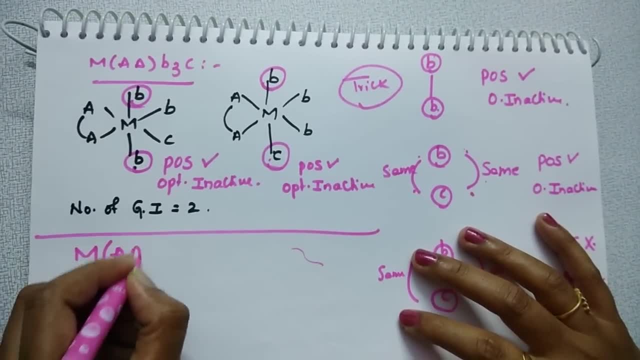 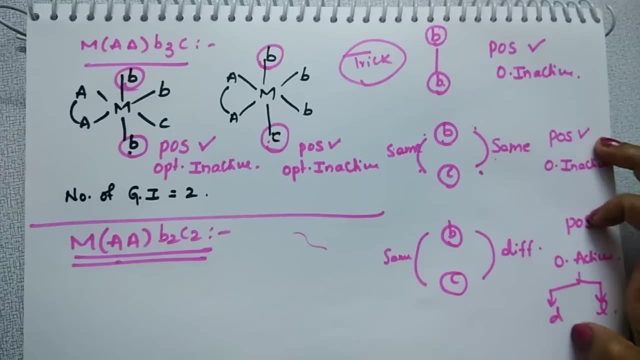